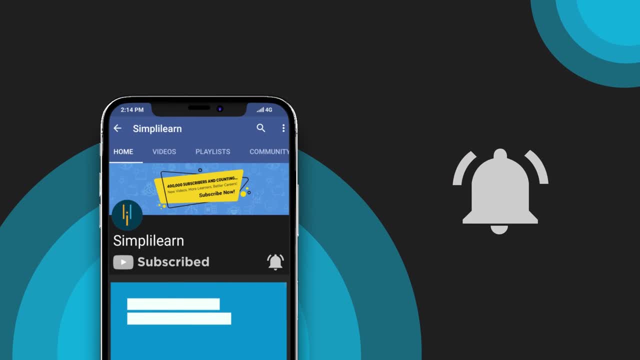 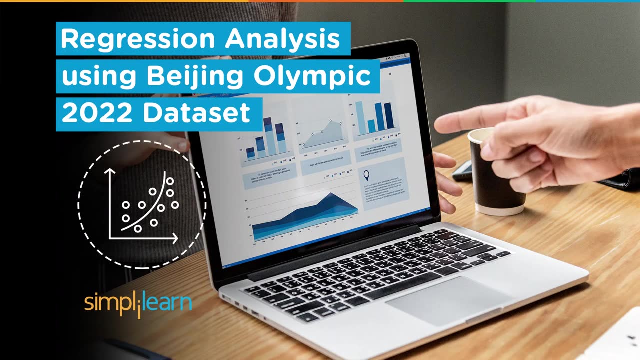 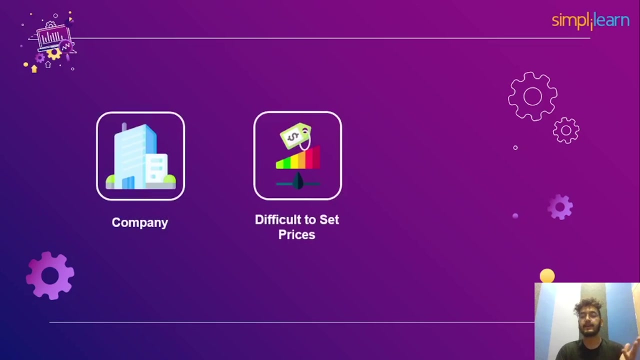 Do you know, in business, it's always been difficult to set the right price for goods or services. Everything is dynamically priced these days, whether it's a movie ticket, a flight ticket, a hotel room or a cafe. Predictive analytics is a common tool, businesses. 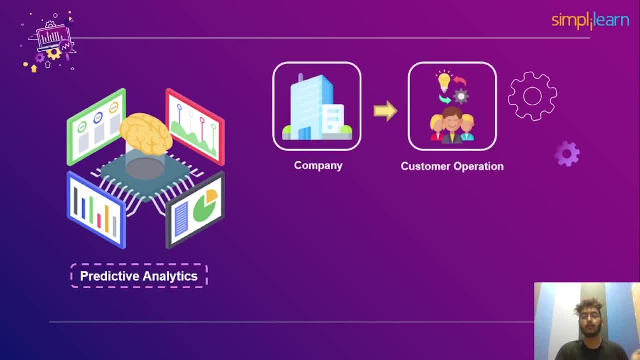 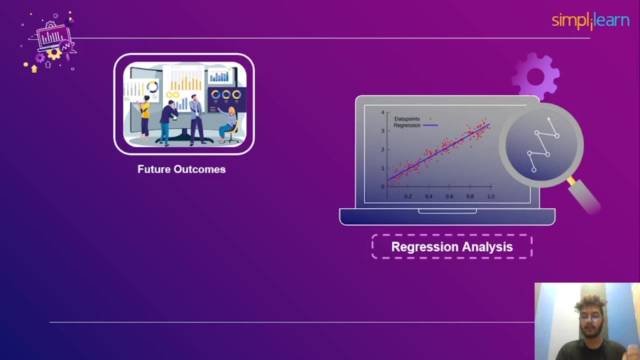 use to target customers and improve operational outcomes. Predictive analytics is widely used in various industries like marketing, manufacturing, real estate, healthcare and many more, In order to predict future outcomes using regression analysis. forecasting consumer behavior is the best use case for the predictive analytics using regression analysis model in the 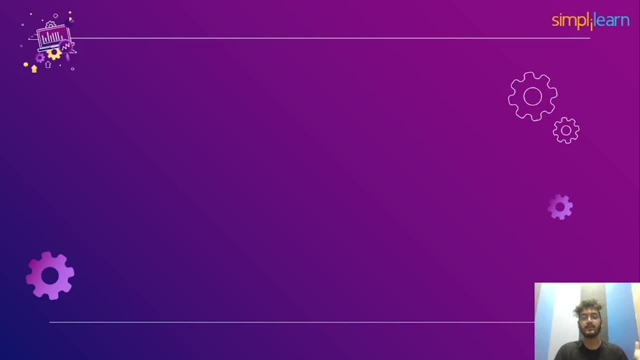 real world. Hey everyone, I am Mayank from Simply Learn. In this video, we will learn what is machine learning, followed by machine learning types. We will continue this session by understanding what is supervised learning, followed by its types. Moving forward, we will look at what 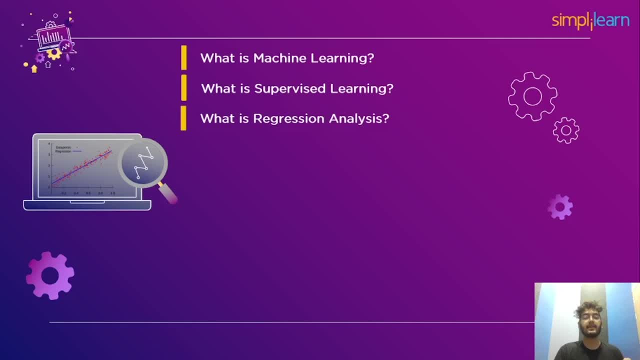 is regression analysis. We will continue this session by understanding why we need regression analysis. After that, we will look at the advantages and disadvantages of different types of regression analysis models. Further, we will also see some popular regression analysis algorithms in detail, followed by application of regression. 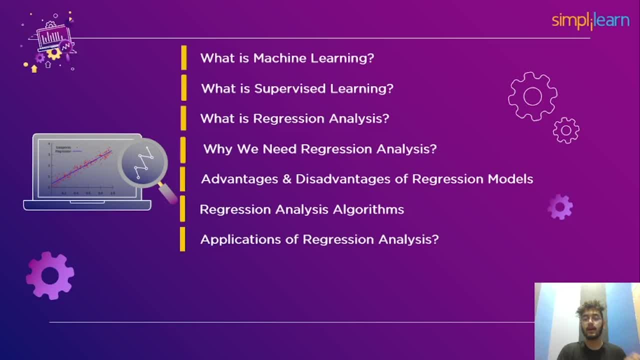 analysis. After discussing regression algorithms, we will see our hands-on lab demo using Olympic 2022 dataset and how regression algorithms work. At last, we will end this video by discussing job opportunities in regression analysis, But before we begin, if you haven't subscribed, 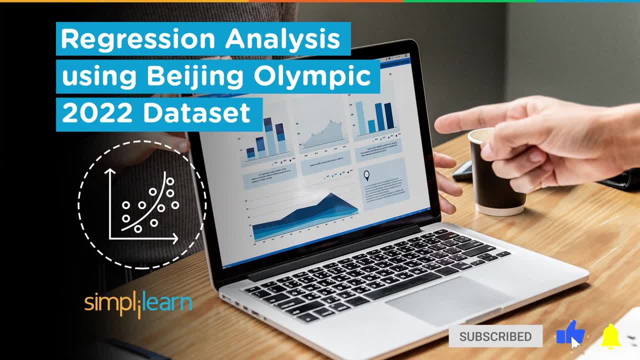 to our channel, hit the subscribe button and please don't forget to press the bell icon so you will never miss any update from Simply Learn. Also, if you are willing to learn more, please subscribe to our channel and hit the bell icon, so you will never miss any update. 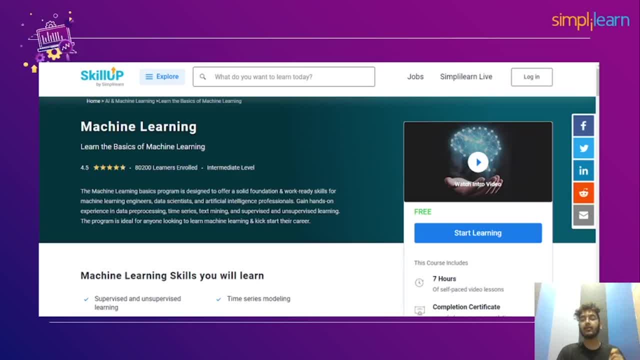 from Simply Learn. Also, if you are willing to learn more about regression analysis, you can check our free course on machine learning by SkillUp as well as the link is in the description. So, without any further ado, let's begin. What is Machine Learning? 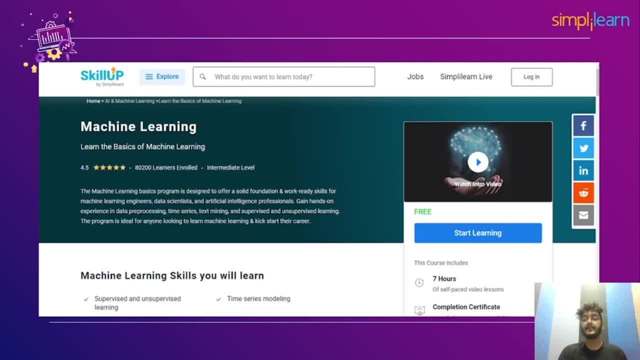 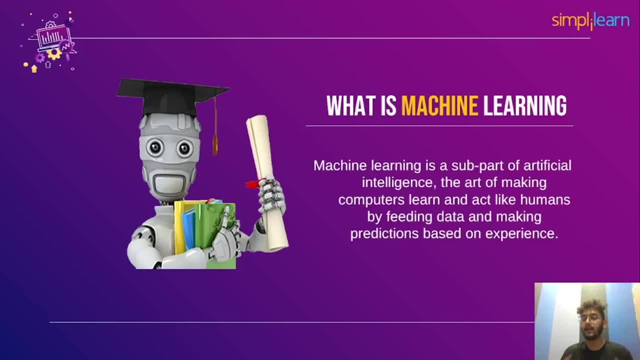 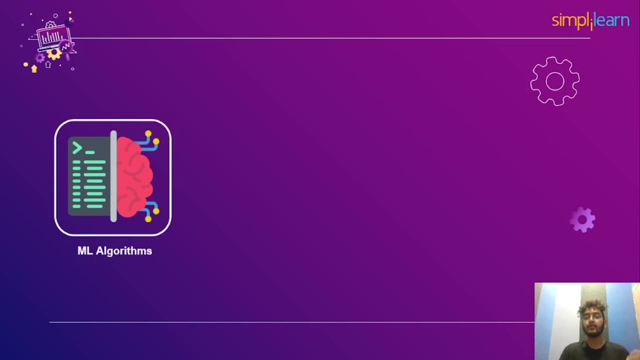 Machine learning is a sub-part of artificial intelligence, The art of making computers learn and act like humans by feeding data and making predictions based on experience. For example, by using ML algorithms, you can determine the quickest route with the least amount of traffic, arrival time, the pickup location and the best optimal information. 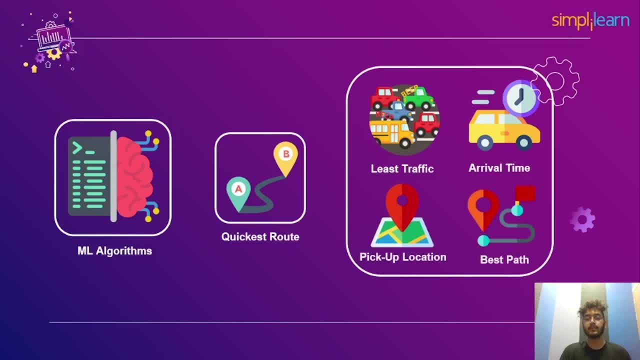 at a certain time and place. However, there are also other types of algorithms that can be used to determine the quietest route, For example, the retrieval route, the pick-up route and the maximum value of a taken part to their destination. 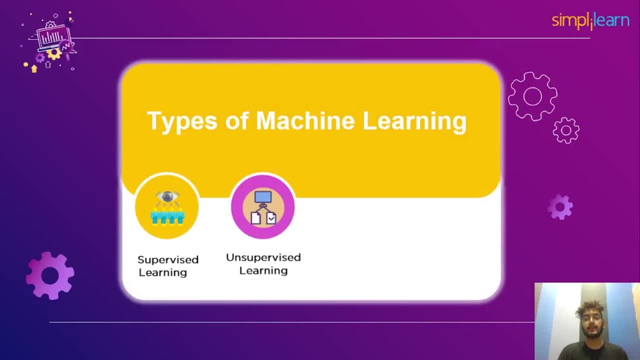 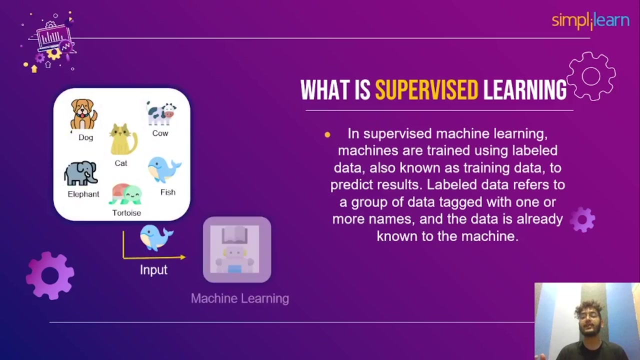 Machine learning is classified as supervised learning, unsupervised learning, reinforcement learning, semi-supervised learning. After understanding what is machine learning and its type, let's understand what is supervised machine learning. In supervised machine learning, machines are trained using label data, also known as training. 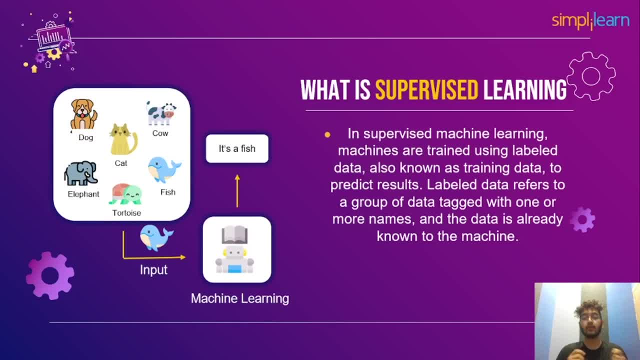 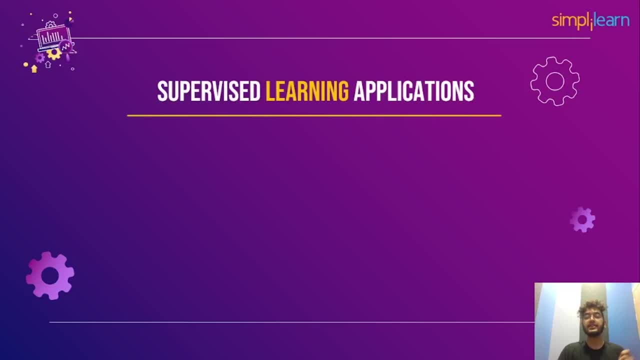 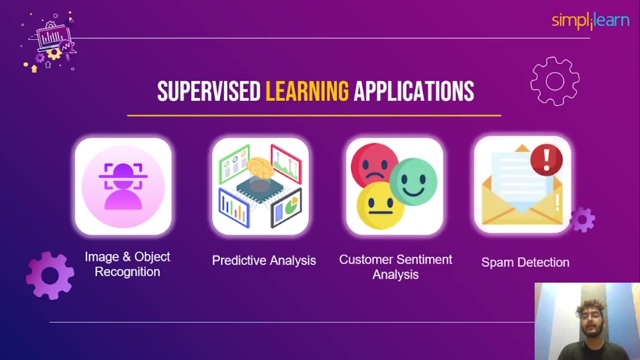 data to predict results. Here, label data refers to a group of data tagged with one or more names and the data is already known to the machine. In the real world, supervised machine learning can be used for image and object recognition, predictive analytics, customer sentiment analysis, spam detection and many more. 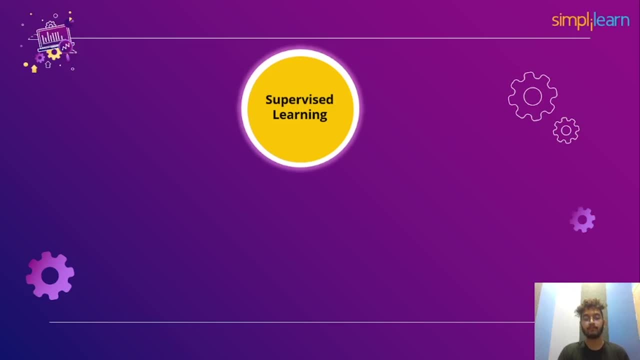 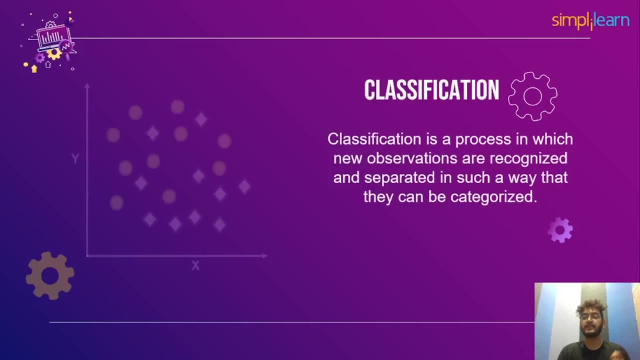 Supervised machine learning can be further classified into two problems, which are classification and regression. Let's quickly understand them one by one. Classification is a process in which new observations are recognized and separated in such a way that they can be categorized. A classification algorithm is trained. 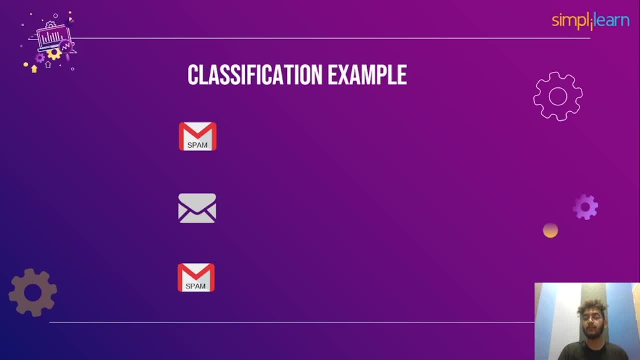 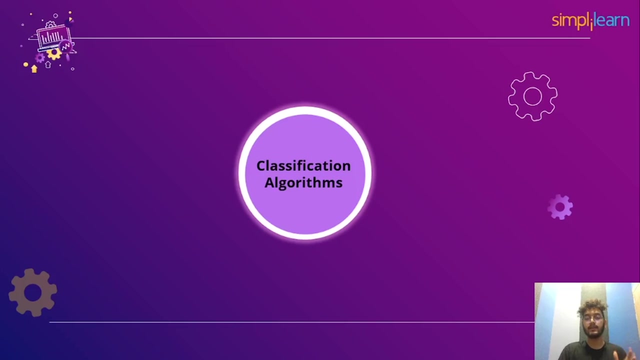 To identify the spam emails by studying the difference between spam and non-spam email. a function that converts an email text into a categorization for spam could serve as a classification model or non-spam classification. There are some popular classification algorithms that come under supervised machine learning. 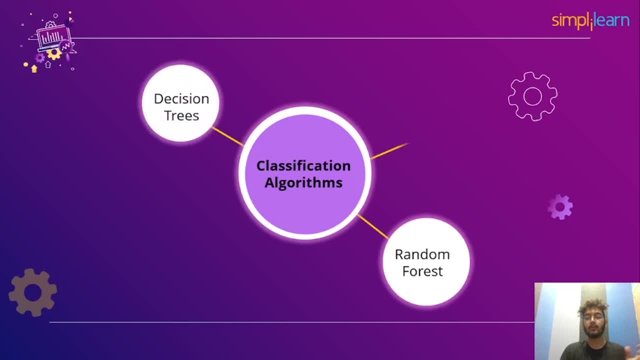 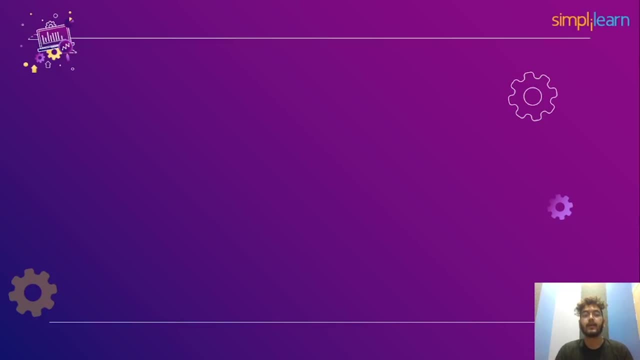 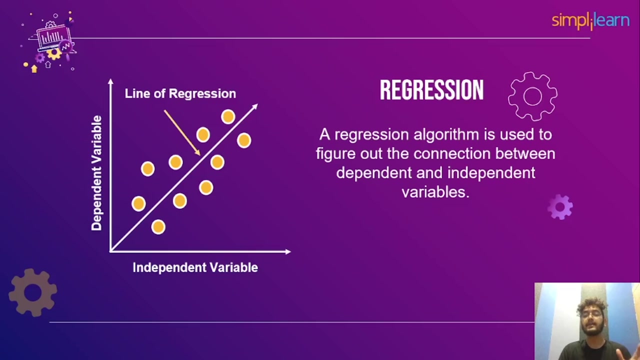 are random forest decision, tree logistic regression, k-nearest neighbors and many more. The next one we have is regression. A regression algorithm is used to find out the connection between dependent and independent variables. Dependent variables are nothing but a variable that we are trying to predict or forecast. 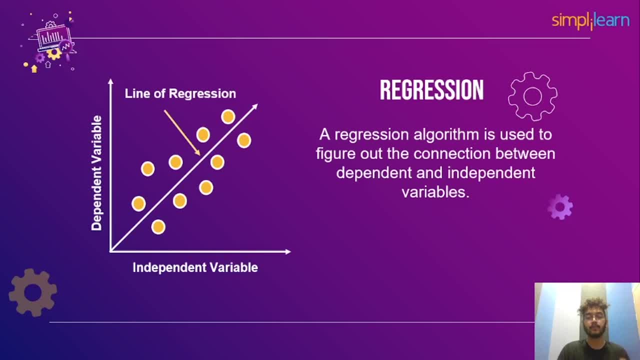 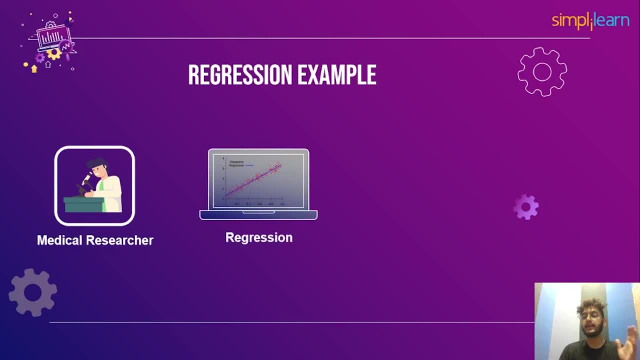 and independent variables are the factors that influence the analysis. It is usually used to make projections. Medical researchers frequently utilize linear regression to study the connection between patient blood pressure and dosage. Researchers may give patients different quantities of a specific medication and track how the blood pressure changes. 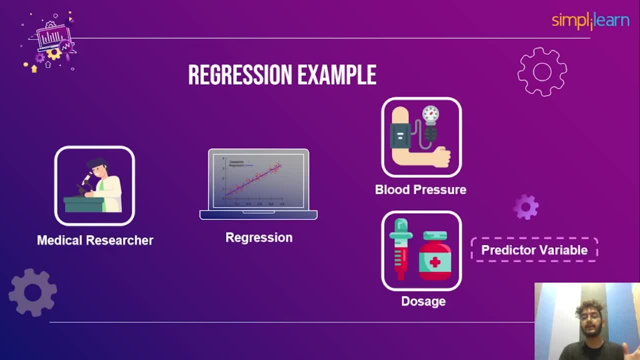 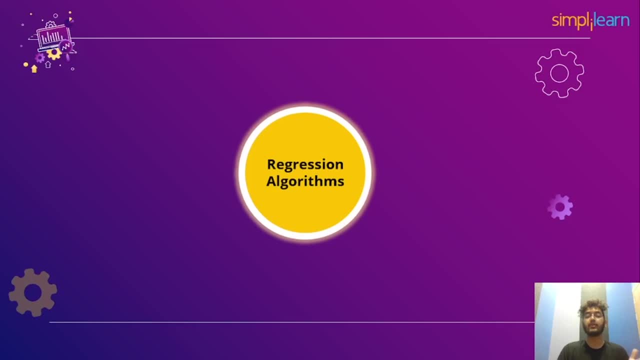 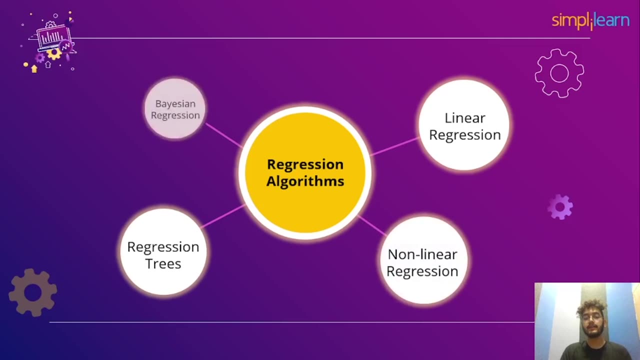 A regression model might use dosage as a predictor variable and blood pressure as a response variable. There are some popular regression algorithms that come under supervised machine learning. First one is linear regression, regression trees, non-linear regression and basal linear regression. After discussing what is supervised learning and its types, let's move forward to see. 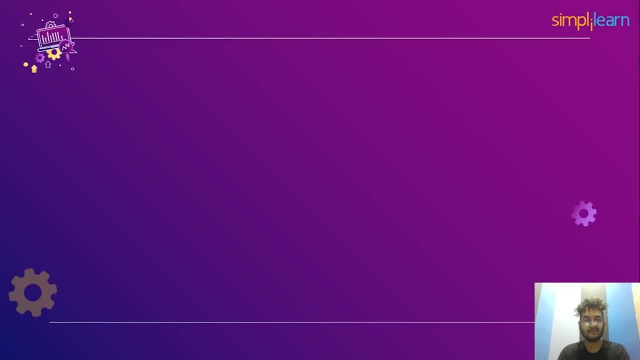 what actually regression analysis is. A static technique is a method of analyzing the blood pressure and dosage of a patient. This method is called linear regression. It is a method of analyzing the blood pressure and dosage of a patient. A static technique known as regression analysis is used to simulate the relationship between 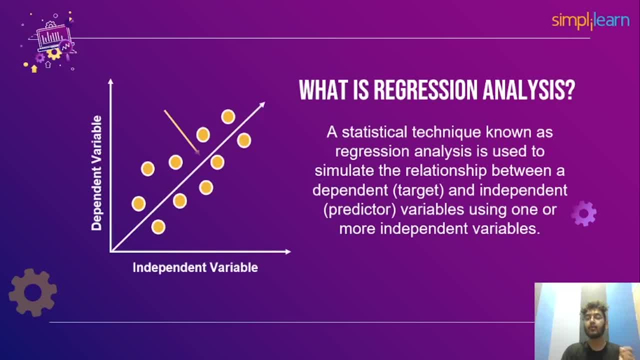 dependent and independent variables. using one or more independent variables, Regression analysis more precisely enables us to comprehend- and when other independent variables are held, constant Changes in the dependent variable values that correspond to an independent variable are changing. Predictions include values that are continuous or real, such as temperature, age, pay and 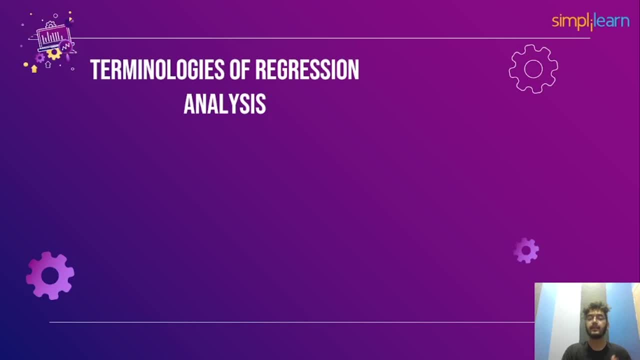 cost. There are some following concepts or terminologies that must be understood in order to completely grasp regression analysis. The first is dependent variable. In a regression analysis, the primary variable we wish to predict or comprehend is the dependent variable. Here dependent variables are also known as target variable. 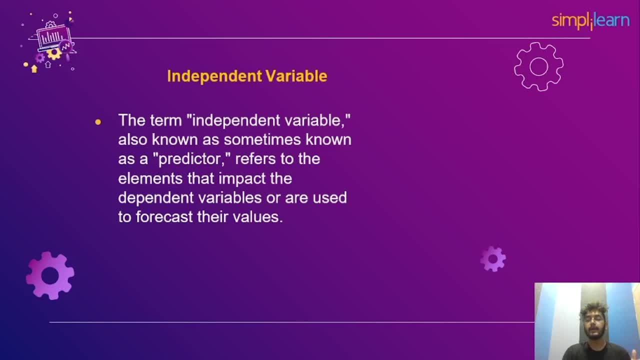 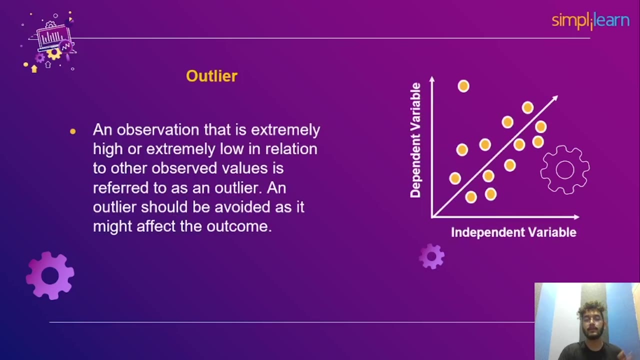 The next one is independent variable. The term independent variable, also known as predictor, refers to the elements that impact the dependent variable or are used to forecast their values. And the third one is outliers. An observation that is extremely high or extremely low in relation to the other observed values is referred as an outlier. 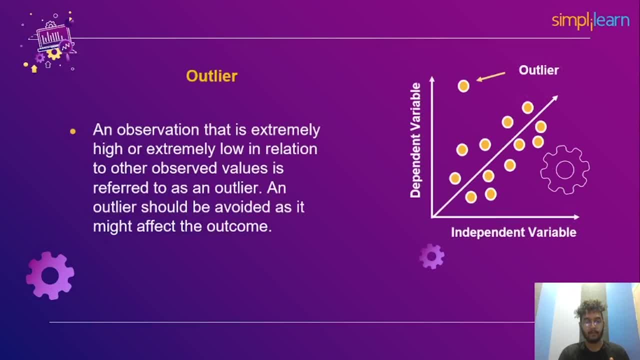 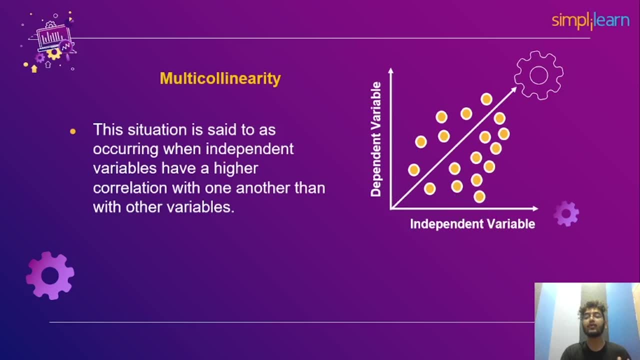 An outlier should be avoided as it might affect the outcomes. The fourth one is multicollinearity. The situation is said to be occurring when independent variables have a higher correlation with one another than other variables. It shouldn't be included in the dataset because it causes issues when determining which variable has the greatest impact. 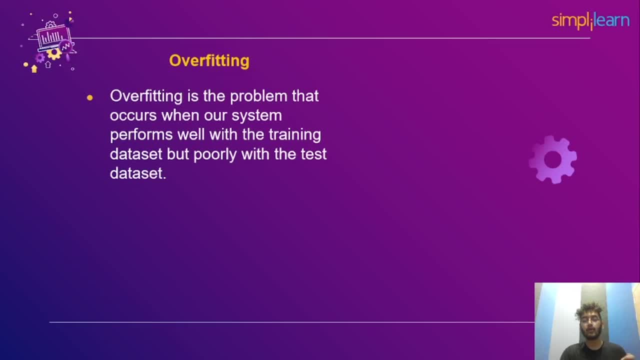 And the fifth one is overfitting and underfitting. Overfitting is the problem that occurs when our system problems well with the training dataset but poorly with the test dataset. Underfitting is the term used when an algorithm does not perform well even with the training dataset. 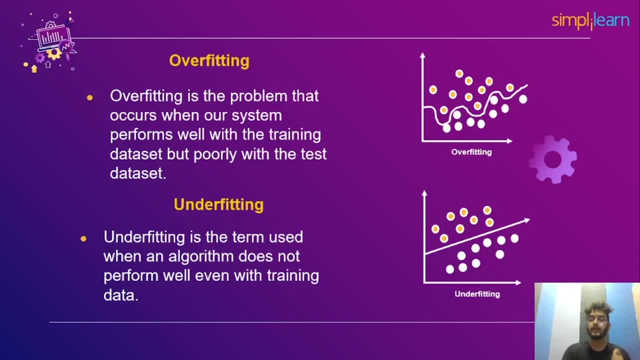 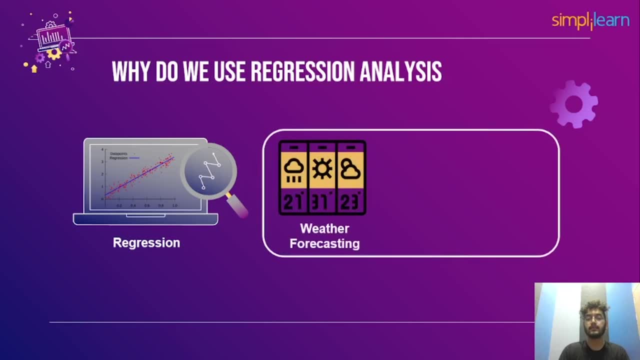 After understanding what regression analysis is and its terminologies, let's move forward and see why we use regression analysis, Including those involving the weather, sales, marketing trends and other factors. in this situation, we need regression analysis that can make forecasts more precise. 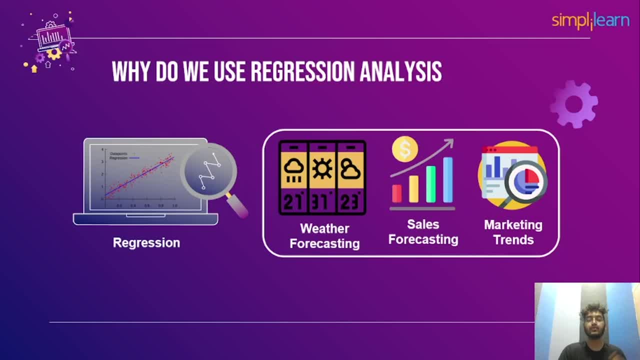 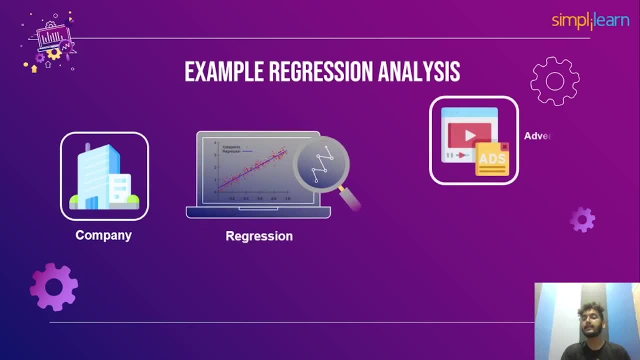 So let's understand the concept of regression analysis using an example. Businesses frequently use linear regression to understand the relationship between advertising spending and income. For instance, they might run a simple linear model with advertising as a response variable and revenue as a prediction. 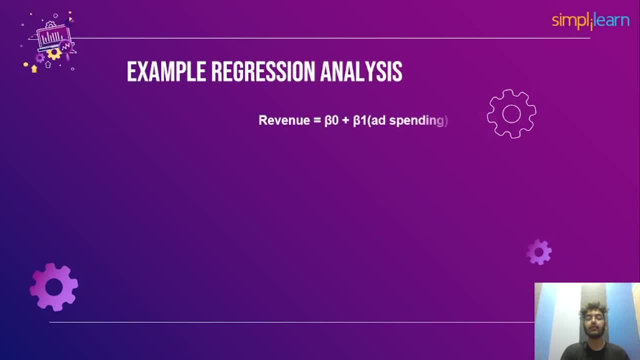 The regression model would look like this: The when equals to beta 0 plus b1 is ad spending. Where there are no advertisements, the coefficient 0 would indicate the whole expected revenue. When advertising expenditures are increased by one unit, the coefficient will represent the typical change in the total revenue, ie $1.. 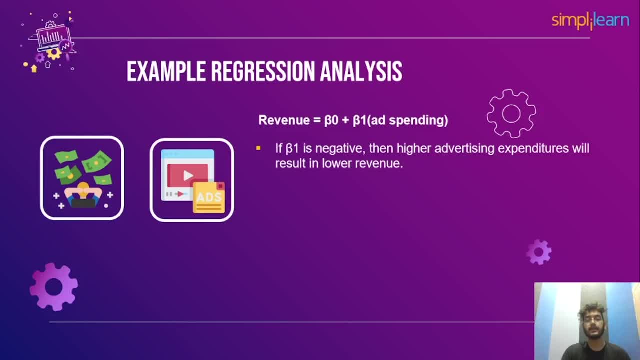 If beta 1 is negative, then higher advertising expenditures will result in lower revenue. If beta 1 is nearly zero, advertising expenditures have leverage. This will have a little impact on revenue, And if beta 1 is positive, it would imply that more advertising expenditures are linked to higher income. 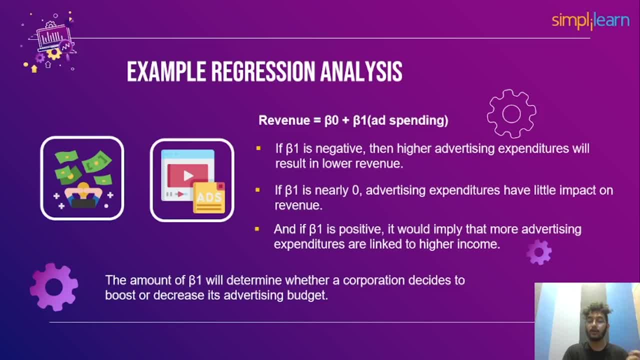 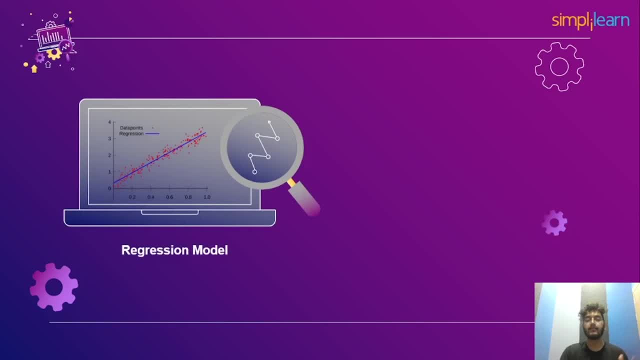 The amount of beta 1 will determine whether a corporation decides to increase or decrease its advertising budget. Regression means creating a graph that connects variables that best fit the given data point. The regression analysis model can then make predictions about data using the plot. Regression analysis is a model of regression analysis. 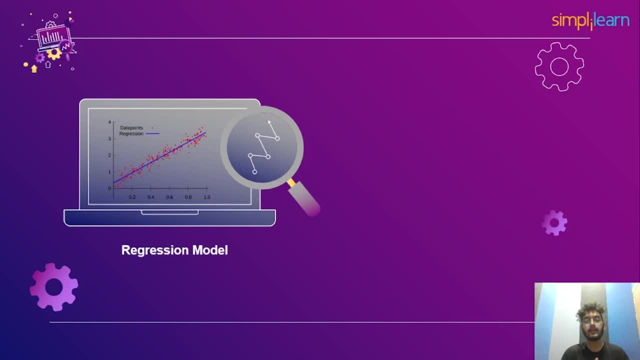 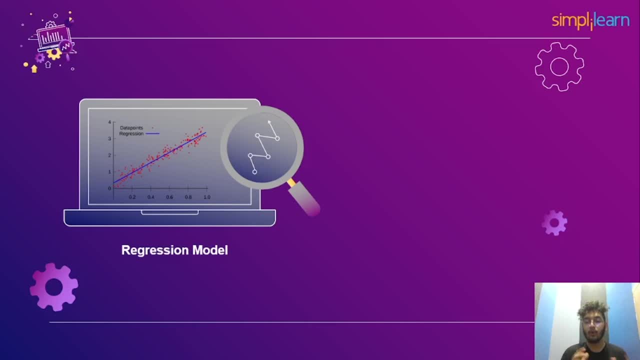 regression is smallest Whether a model has captured a strong link between, determined by the distance between data points and the line. There are some more use case of regression analysis, like we can use temperature, another variable, to predict or forecast rain. Regression analysis can be used for identification of market trends, For predicting traffic accidents caused by reckless 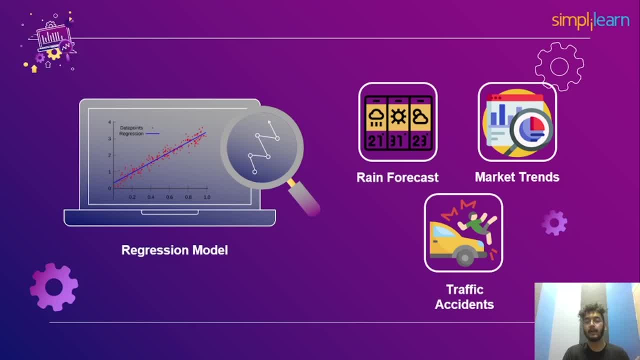 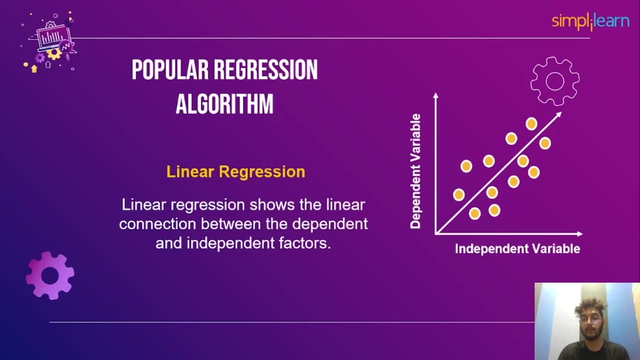 driving. we can use regression analysis for the same and many more. So, by understanding why we need regression analysis, moving forward, let's see some popular regression algorithms in detail. The first one is linear regression. Linear regression is one of the most famous and straightforward machine learning algorithms utilized for predictive analysis. Linear 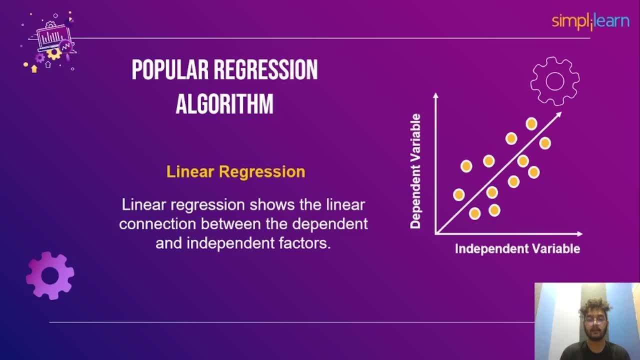 regression shows the linear connection between dependent and independent factors. The line of the equation is: y goes to mx plus b. Here y stands for the response variable or a dependent variable, whether x is for the predictor variable or an independent variable. Here m is the estimated slope and b is for 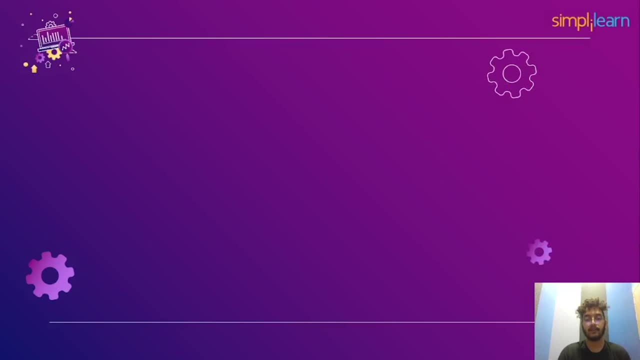 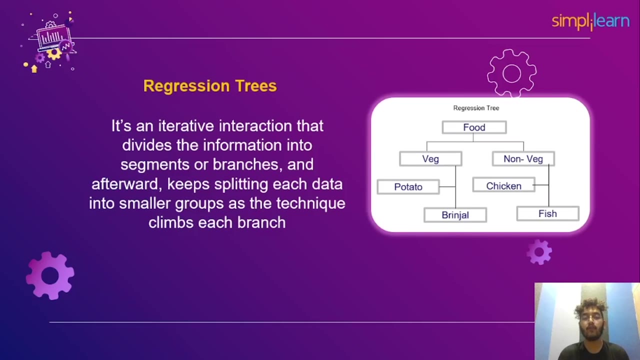 the estimated intercept, And the next one is regression trees. A regression tree is worked through a cycle known as binary recursive, which is iterative interaction that divides the information into segments or branches and afterward keeps splitting the data into smaller groups As the technique climbs each branch this tree is used for. 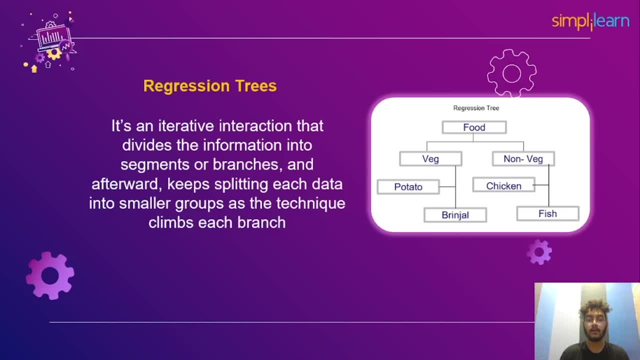 the dependent variable which continues values. For example, a regression tree is named food, which is divided into segments: veg and non-veg. Further, it keeps splitting into smaller groups. And the third one is nonlinear regression. Nonlinear regression is a type of regression. 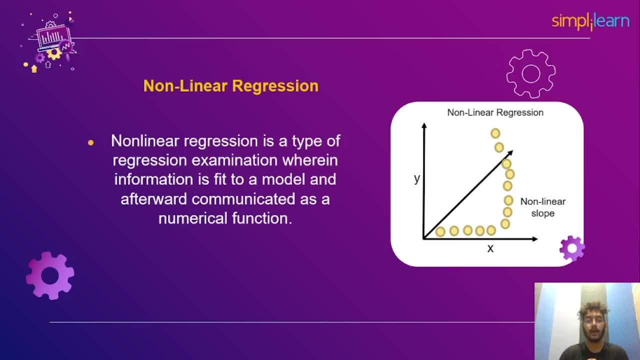 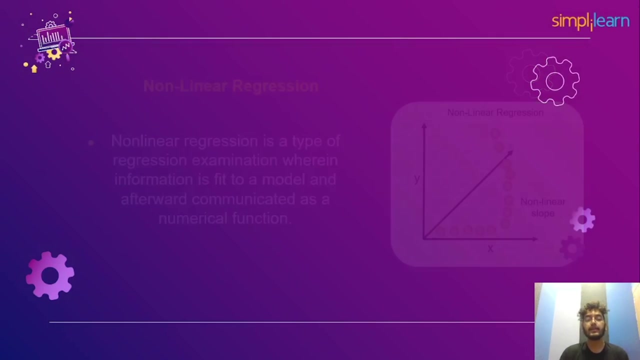 examination wherein information is to pit a model, And, after the regression is completed, the data is then split into segments or branches. And the next one is linear regression. Nonlinear regression tells us about the relationship between gtp and the country, And the fourth one is Bayesian linear regression. 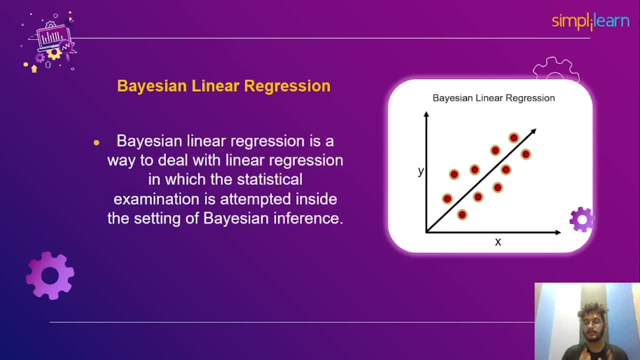 The algorithm is a way to deal with a linear regression in which statistical examination is attempted inside the setting of a Bayesian inference. Linear regression and Bayesian regression can generate the same prediction and with the help of Bayesian processing we can retrieve the complete variety of inferential solutions. 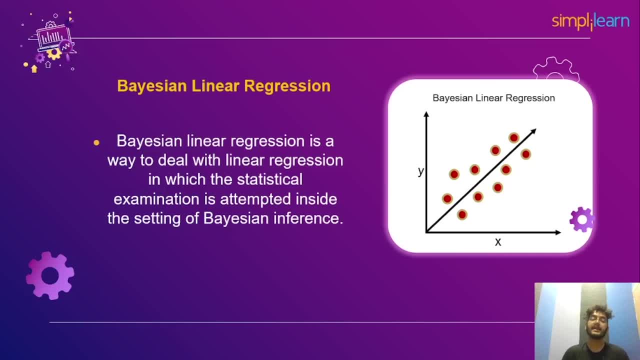 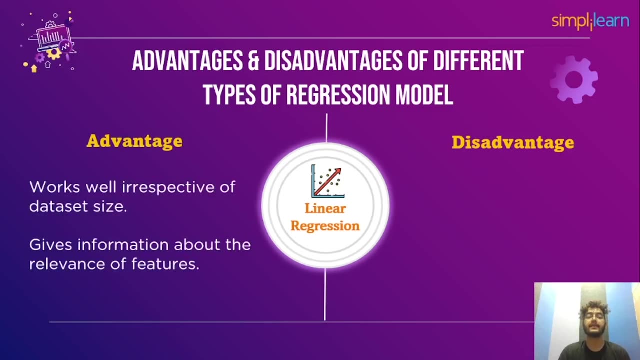 instead of a point estimate. After seeing some regression analysis algorithm, let's move forward and see advantages and disadvantages of different regression analysis models. And the first model is linear regression model. The advantages are: work well irrespective of data set size. and the second one is gives. 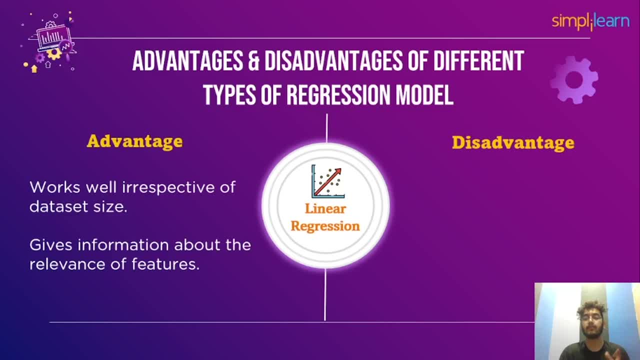 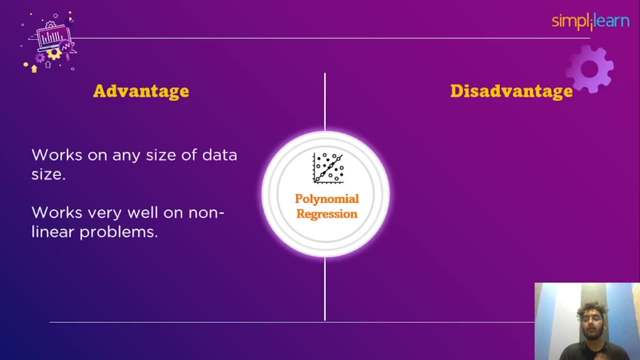 information about the relevance of features and the disadvantages are the assumptions of linear regression and the next one is polynomial regression. The advantages are works on any size of the data set and the second one is works very well on non-linear problems. and disadvantages are we need to choose the right polynomial. 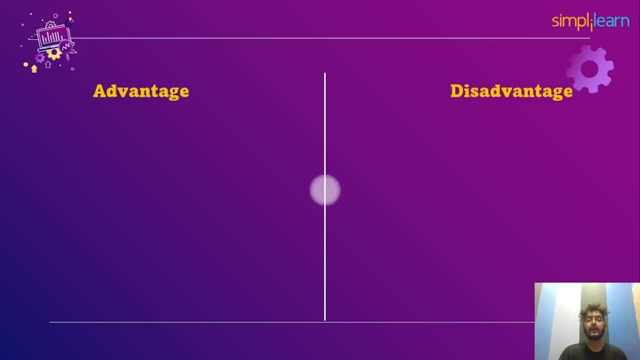 degree for the variance trade-off. The next one is support vector regression algorithms and the advantages are easily adaptable, works very well on non-linear problems, And disadvantages are difficult to understand and not well known. And the next one is decision tree regression. The advantages of decision trees are no need to apply scaling and the second one is works. 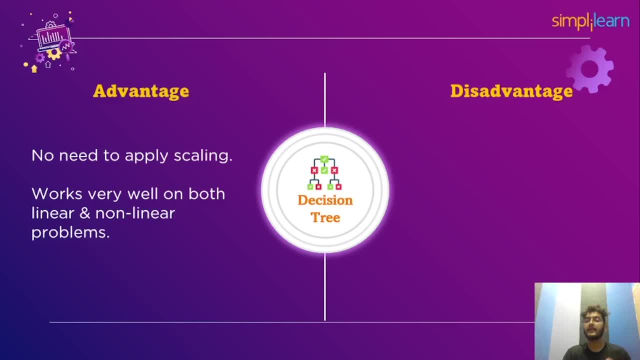 very well on both linear and non-linear problems, And disadvantages are poor results on a small data set and overfitting can easily occur. And the last one is random forest regression. The advantages are powerful And second one is accurate And disadvantages are no interpretable. and the second one is: overfitting can easily occur. 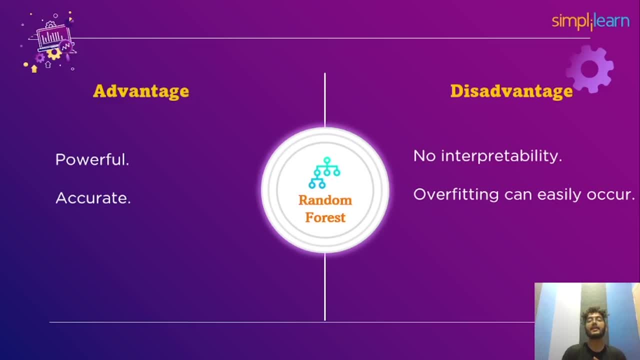 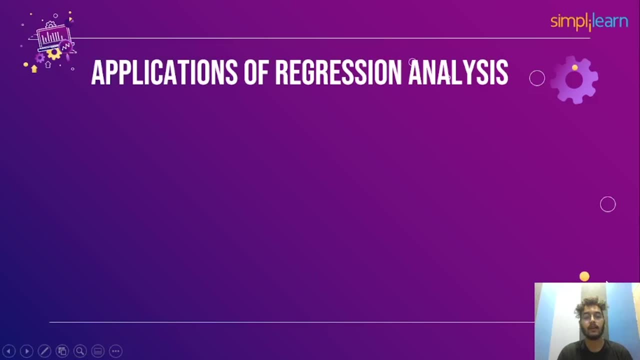 After seeing advantages and disadvantages of different types of regression analysis models, let's move forward and see some applications of regression analysis. The first one is forecasting. Regression analysis is frequently used in business to predict potential opportunities and dangers. For example, demand analysis predicts how many items a buyer is likely to buy. 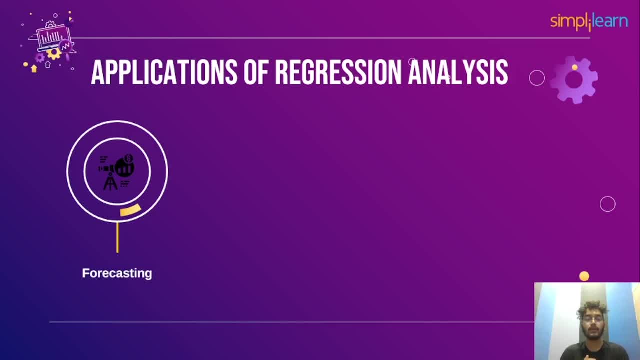 For example, demand analysis predicts how many items a buyer is likely to buy. For example, price is expected to be about 600 dollars every month, which is exactly help. You can pull it out- corporate return and operational performance when doing financial analysis. And the third one is comparing with competition. 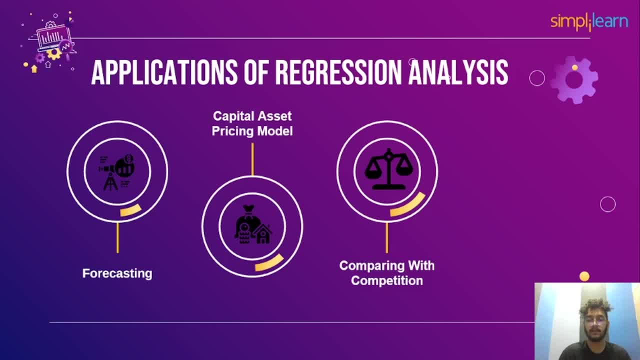 It can be used to evaluate how well a business is doing financially in comparison to a certain rival. It can also be used to figure out how the stock prices of two companies are related to one another. This can be extended to find the correlation between two competing companies. 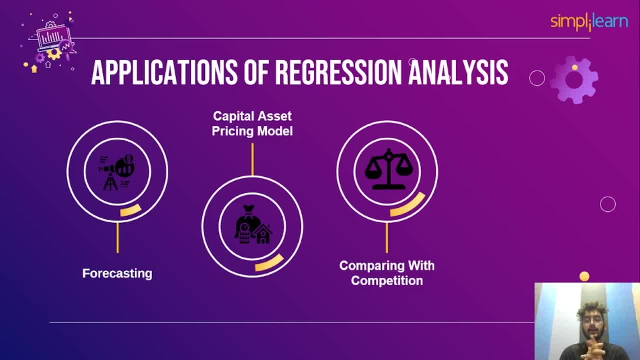 It might help the company in identifying the factors affecting the sales, in contrast to the comparable company. These methods can help small businesses succeed quickly within a short period of time. And the last one is identifying problems. Regression is beneficial for identifying incorrect judgment as well as for providing factual. 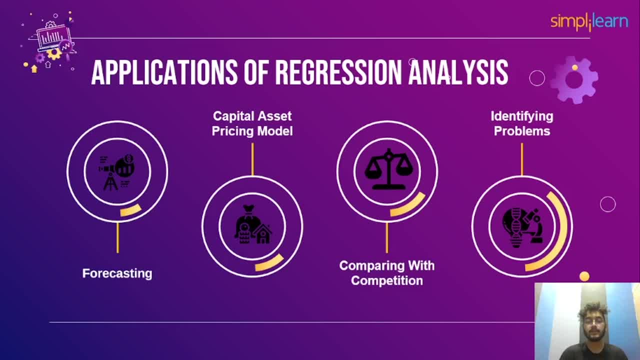 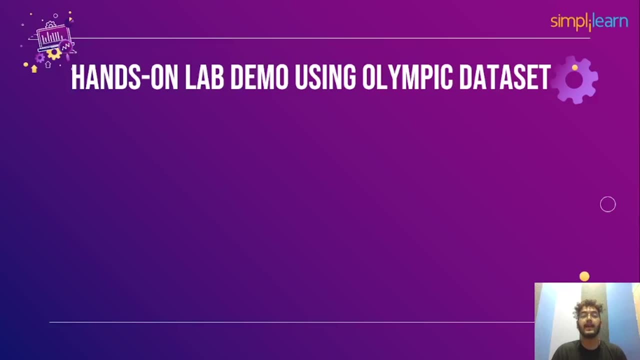 support for the management. For instance, a retail store manager might believe that extending the hours of operation will greatly increase sales. After seeing the application of regression analysis, let's understand the regression analysis using the code. So now we will see hands-on lab demo using Olympic dataset 2022.. 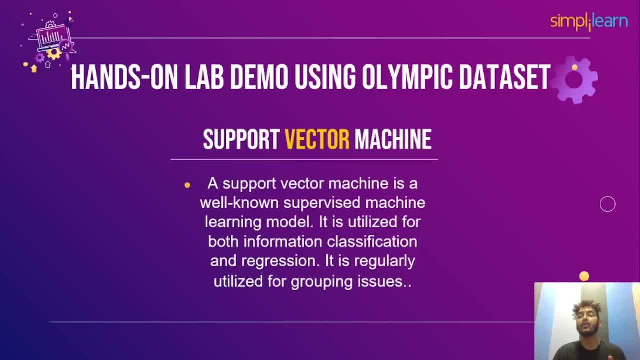 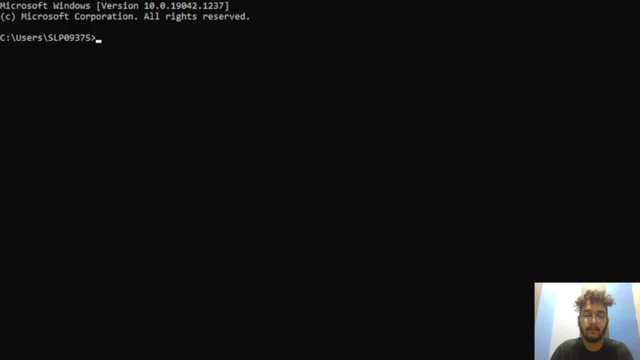 So we will use support vector machine. A support vector machine is a well-known supervised machine learning model. It is utilized for both information classification and regression. It is regularly utilized for the grouping issues. Let's open Jupyter notebook. So this is our command prompt and here we will write Jupyter notebook to open Jupyter. 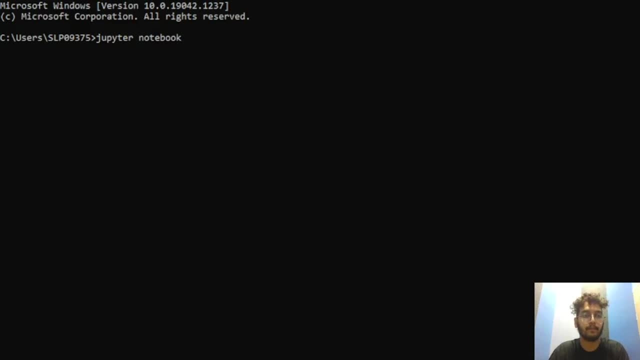 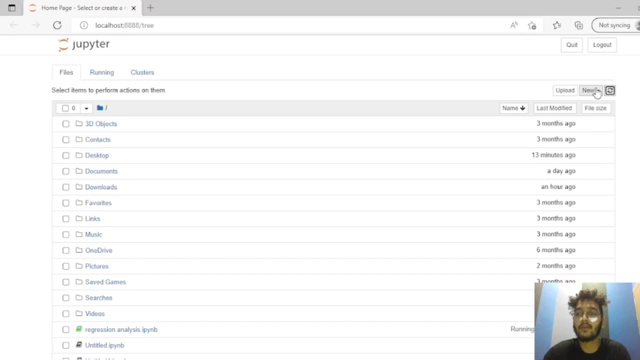 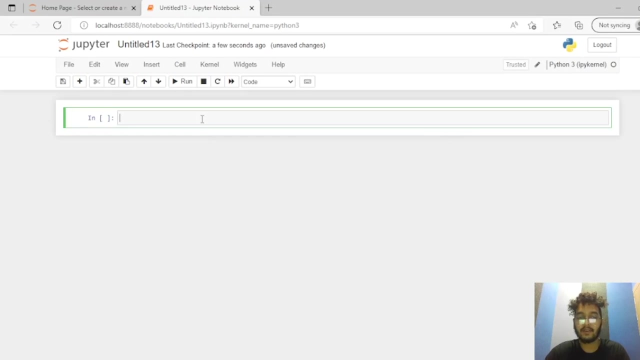 notebook. So press enter, Press enter. So this is the landing page of Jupyter notebook, and here we will open one python file. So this is how the Jupyter notebook UI looks like. So at first we will import some major libraries of python which will help us in mathematical. 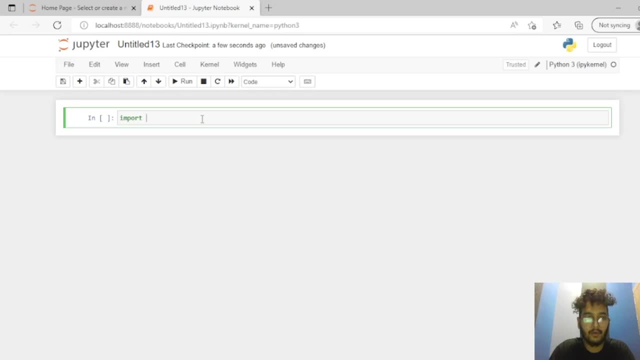 functioning. So the first one is numpy, So we will write import numpy as np And press enter. So numpy is a python library used for working with arrays. It also has function for working in the domain of linear algebra and matrices. It is an open source project and you can use it freely. 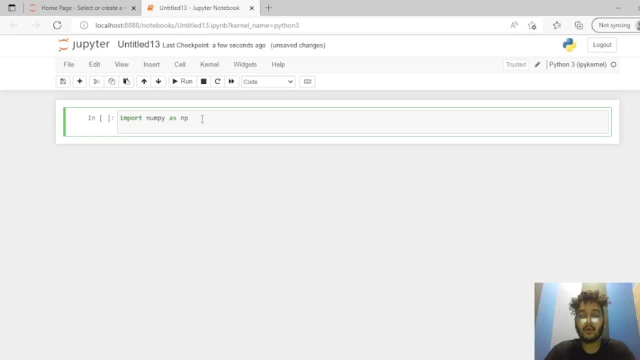 So numpy stands for numerical python. So we will import the next library as pandas. So we will write import pandas as pd. So pandas is a software library written on python programming language for data manipulation and analysis. In particular, it offers data structure and operation for manipulating numerical tables. 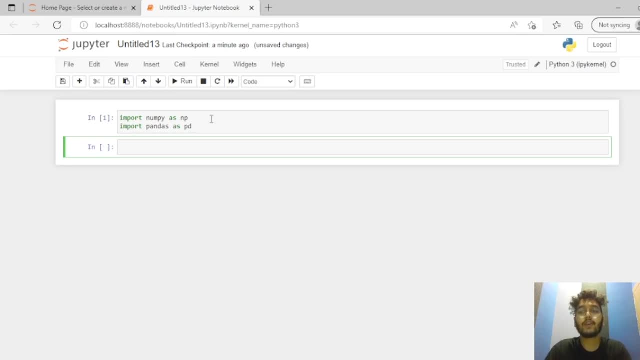 and time series. So after importing the libraries, we will move forward and import data set. So for importing data set we have to write: data equals to pd dot, read underscore csv. So here we have to write our data set name: Ollam. 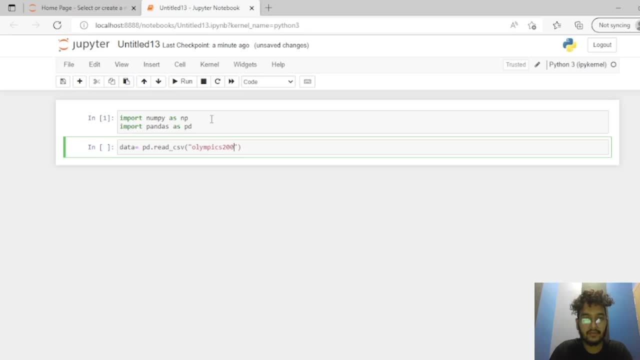 It's csv, So O is capital in my file. so I don't know what's going on. Yeah, perfect, So press enter. So here, pd is for pandas library. Read is used for the reading the dataset from the machine. 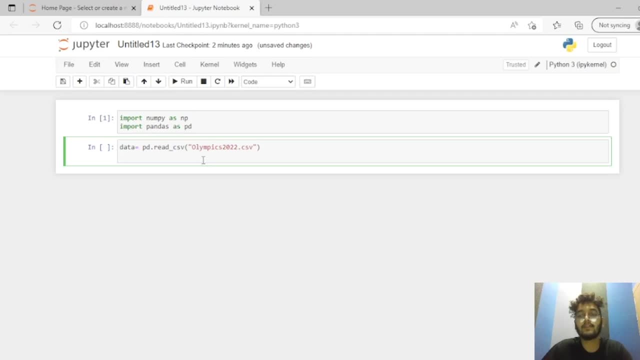 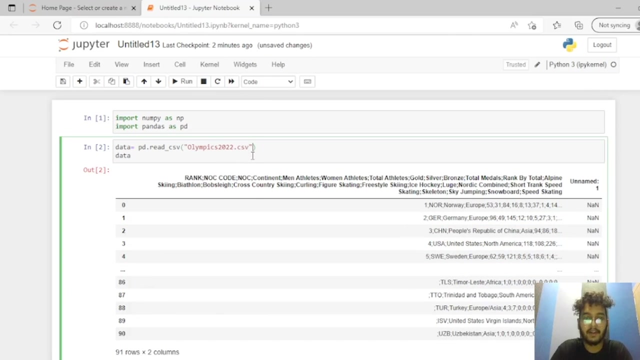 And csv is used for the type of files, So pd, which you want to read. so then we have to write data set data to see our data. so press enter. so this is how our data set look like. so for separating data, like in a proper row, and 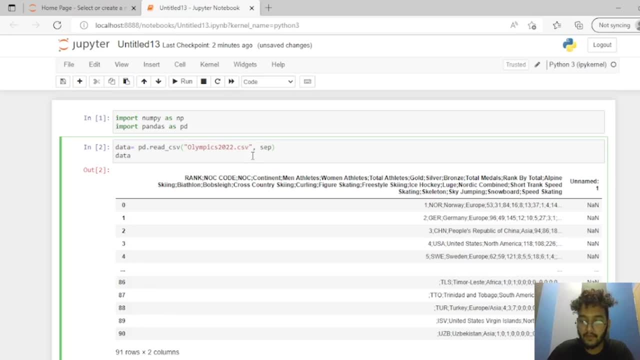 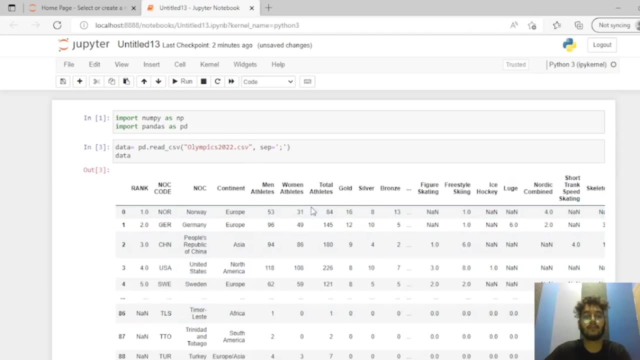 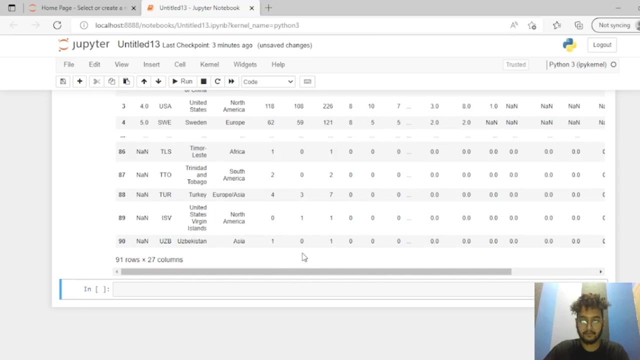 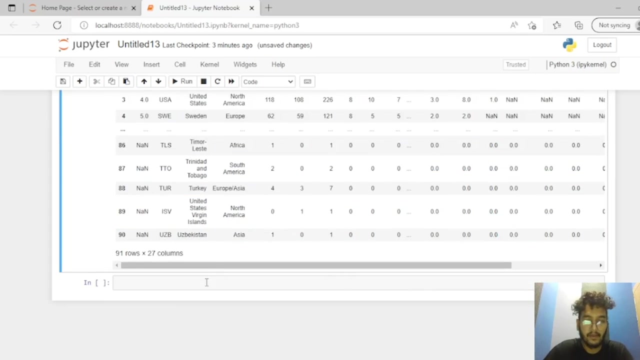 column, so we can use here: sep equals to this semicolon. so after this enter. so this is how our data look like. so this is 91 rows and 27 columns data. so so, moving ahead, we will replace ns values like these: ns values from zero. so we will write here. so we will write here: data equals to. 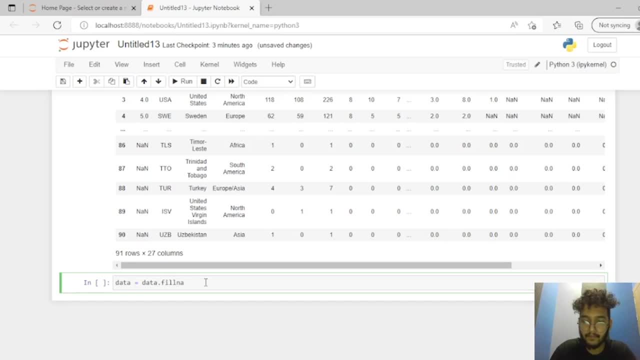 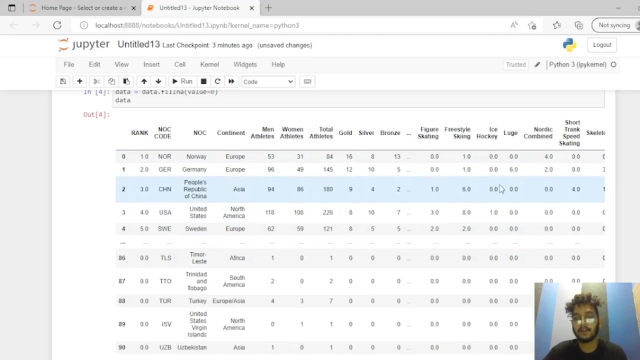 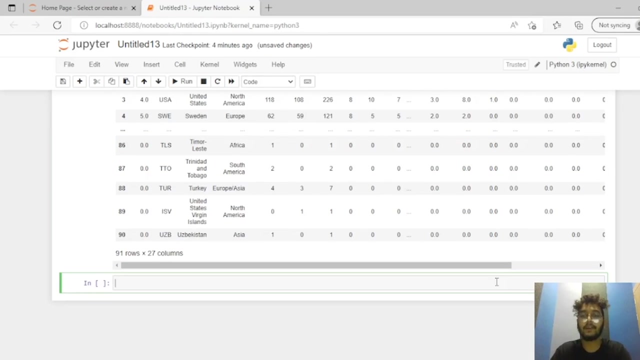 data dot fill na value equals to zero. so after entering, we will write here data and press enter. now see just we have replaced all ns with zeros. for better results, see all zeros with n is here and no n is here. moving ahead now let's see how our data looks like in pie chart. 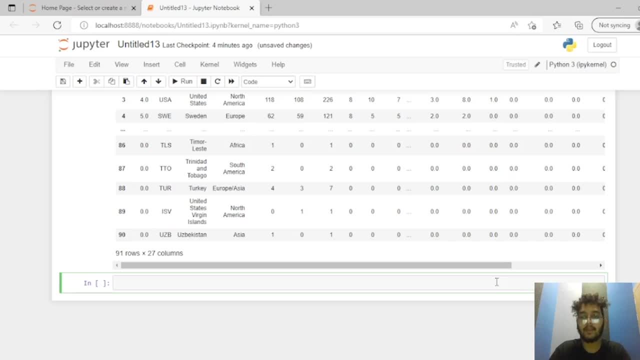 so we will write import some matplotlib libraries. so we will write import matplotlibpyplot splt. so matplotlib is a graph plotting library in python that serve as a visualization utility. matplotlib is a open source and we can use it freely and it is mostly written in python. a few: 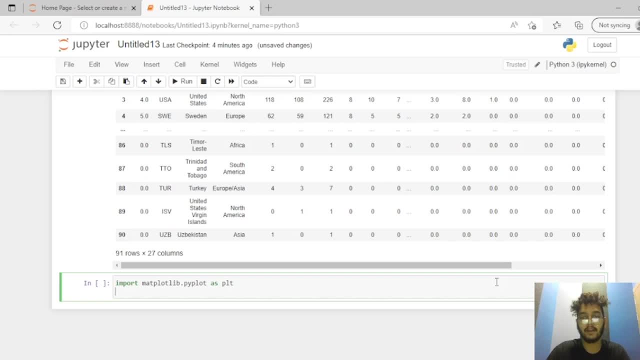 segments are written in c and javascript for platform compatibility. so we will write here some male athletes, oh, athletes, i guess athletes, sorry for that. athletes equals to data square brackets. we have to write men. a capital at leads, so dot sum. so after enterings we have to write sum. 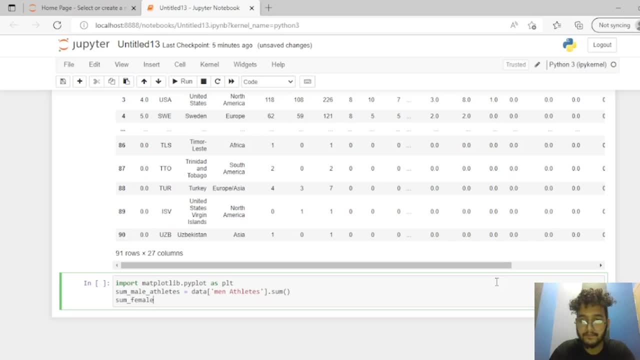 score email underscore: athletes equal to a z in the st certificate. equal vérit natits equal to a z in the test certificate. equal to a z. equal to a z in the test certificate. no, no, we have to write here. so here: equal to delta. equal to: 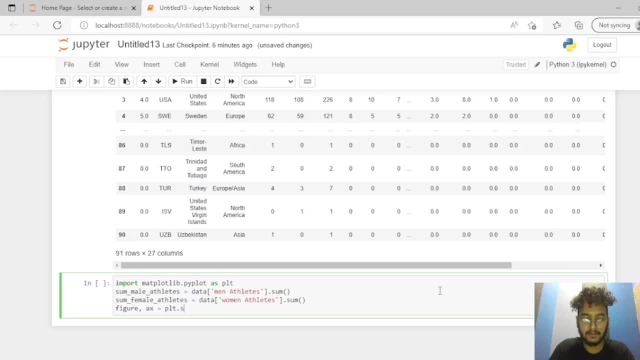 equal to 円, or subplots, the blocks size. oh sorry, bigger size size equals to. you can hear, give 12 comma 6. so so here subplots, like a subplot is a secondary strand of the plot, that is a supporting side story for any story or the for the main story. so we will write here ax dot pi for the pie chart and 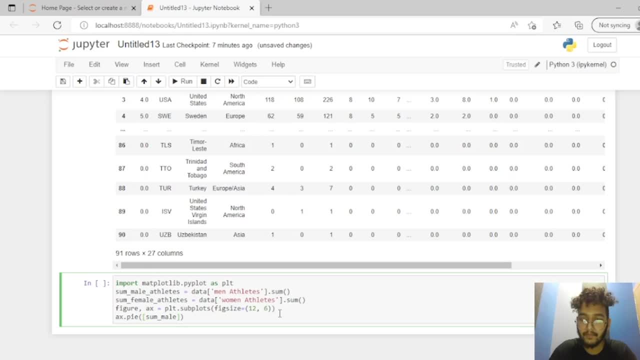 some underscore me: the school athletes comma. right, here's some underscore female score at least square bracket comma text props goes to the city, or the color of woman was to W, so like we have to give your legends a dot legend. oh men, this is for men. comma woman. so 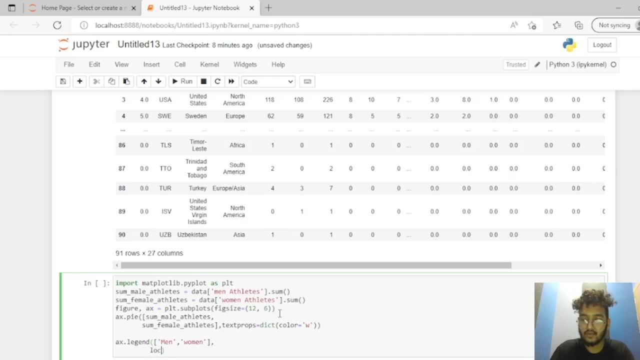 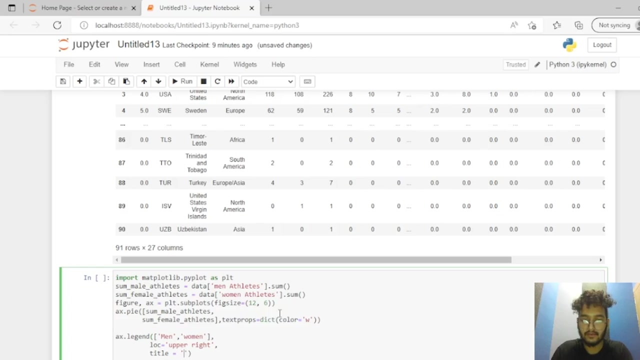 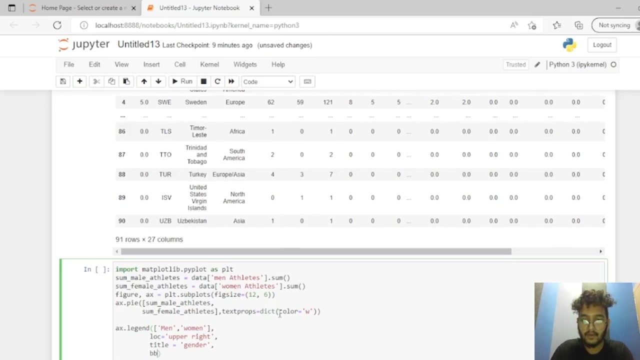 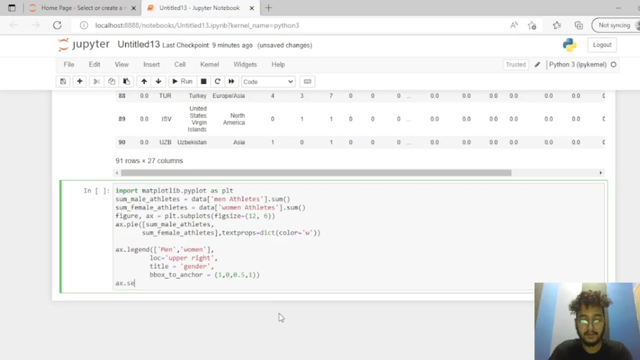 so LOC was to upper right comma title title equals to gender comma, maybe, Oh X, and let's go to, and this is for just a change, equals to: you have to give here one comma like zero comma, zero point four, five here, give one. so let's keep in. type is so. we will write here: ax dot set title title. so here we can. 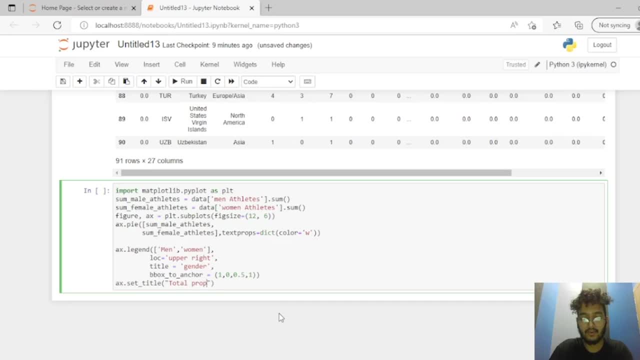 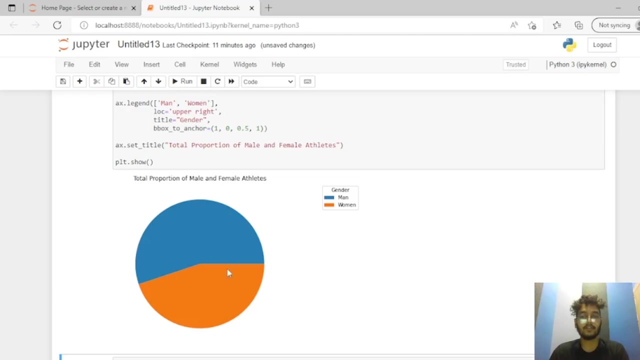 give title like total proportion of of male and female. N learn at home between a忍者 off of male and female athletes. so after this we can write PLT dot show. we can here write PLT dot show and we will see now like how our pie chart look like. so so this is how our pie chart look like. 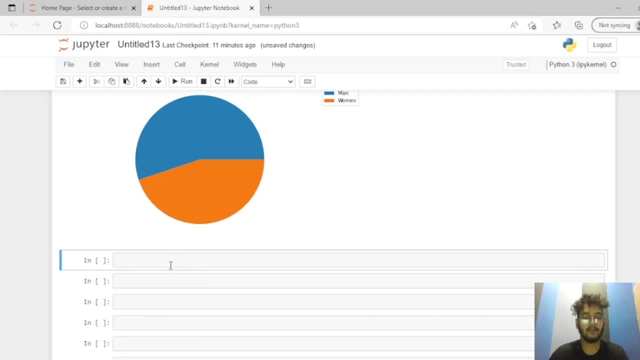 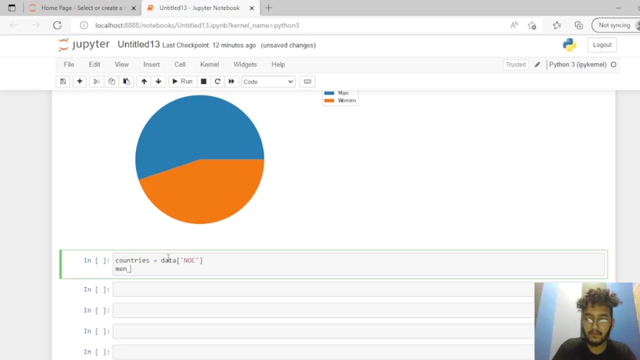 so, moving ahead, let's see one more visualization: data with bar graph. so we will write here: countries- countries equals to data NOC. we have to just write in. so we will write here: men underscore athlete equals to data NOC. so we will write here: men athletes go. women underscore athletes equals to data: women athletes. 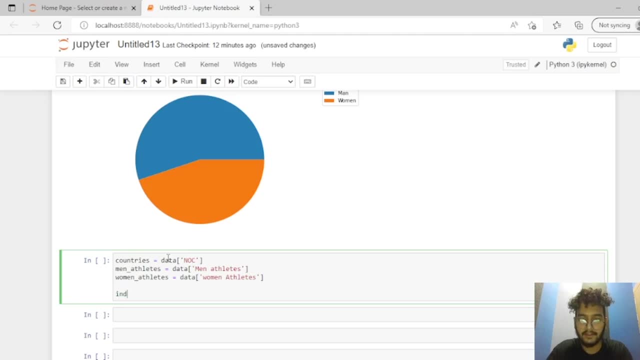 here we will write: INT equals to NT, dot, arrange, arrange. so we have to give here length, len. so countries, countries, countries, countries, countries, countries. okay, into we will write 32 here. so width, we will give width, we will give maximum width, we will give 8, it's your wish how much you will give. so here we will write figure comma. 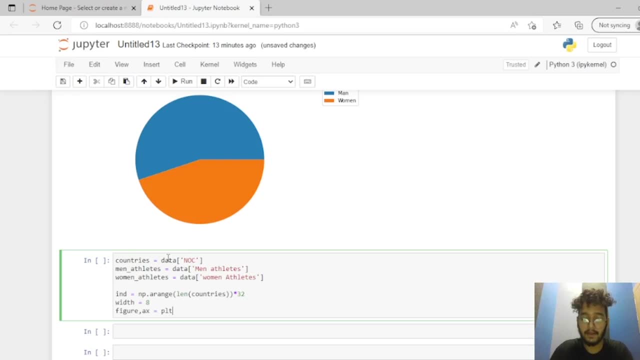 AX equals to ELT dot subplots, subplots. so here we will write 32. here we will write 32: plot続 rid cycling, 論 64.60. we will write ax dot bar, because we are creating bar chart here, so we will write: 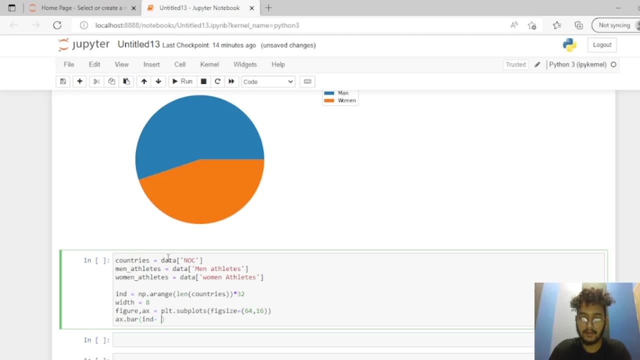 INT which is: width, ΔAbike .2.2 DC. current result: come on, man, man, and she leads. come up with, goes to: first we will write a date again. well, it was two men, perfect. so here again we will write a s? dot, but I am D plus with where the bed to come on, man, at least. 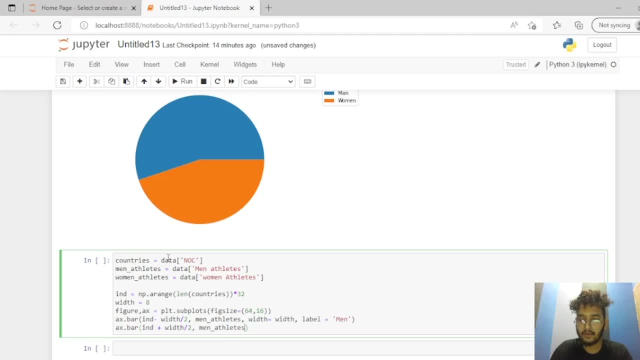 so so write not. then this time we have to right woman, woman, you, so let come out of this. so here we will write ax dot set. we have to set the y label and the x label. so first we will write for the y label, so available. so this is like amount, comma, font size. 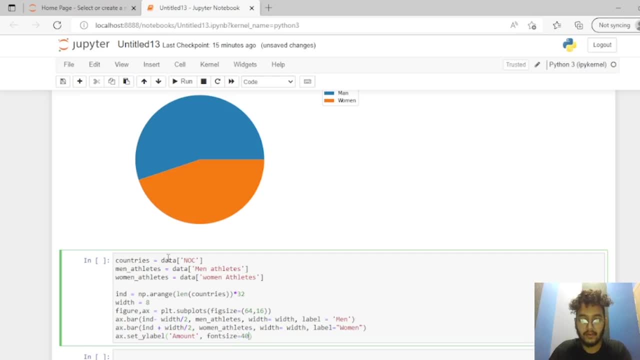 equals to 40. so ax dot set title. we will write the title. but we will give like title, like male and female athletes from like we can use different, different countries. so comma: font size equals to. font size equals to. we will write 0.50. so. 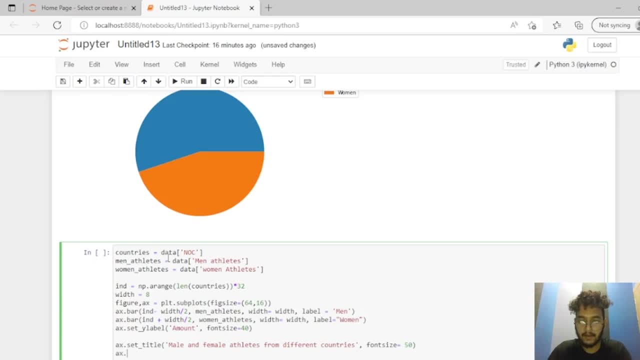 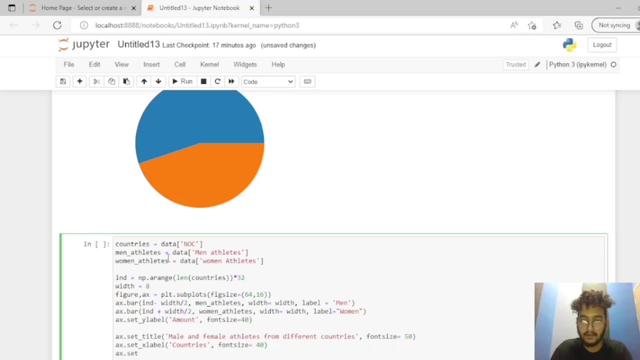 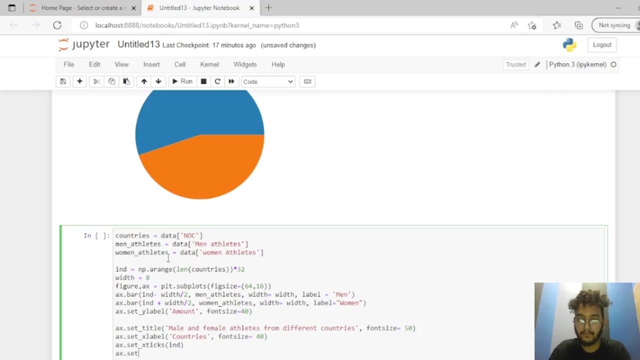 like this. so let's set the x labels so underscore label, sorry, x label. so here we will write: countries size equals to 40: 40. so ax dot set set underscore x ticks nd. so we will write here: ax dot set underscore x ticks, not ticks. you have to write only tick, so labels. 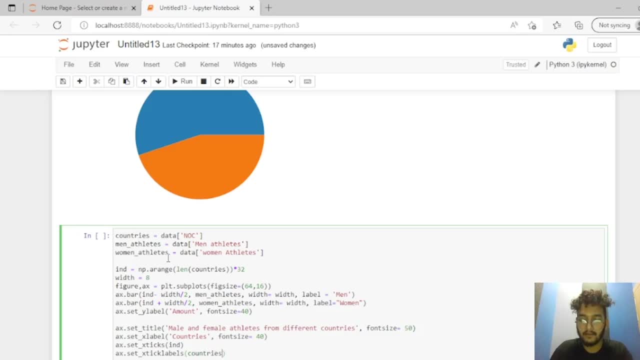 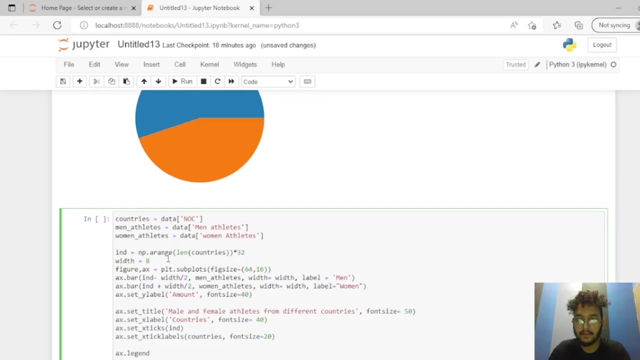 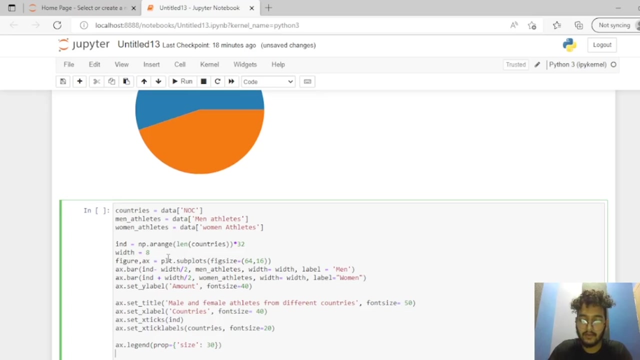 browser please. size equals to 20, so ax dot legend prop equals to size. let us try import from the document tee. enter these two of them. okay, you took it like this on a 30 so you have to write plot PLT dot as it set up. 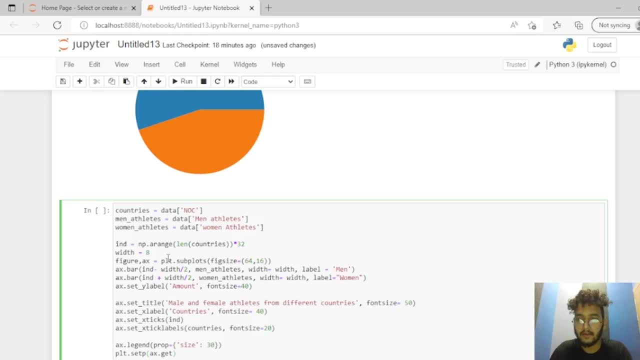 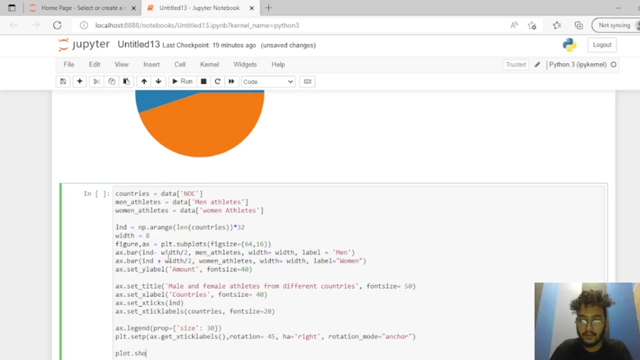 ax, don't get X, click labels and comma rotation equals to 45. so we will write here: h equals to right and again comma rotation underscore equals to anchor. so finally, the time is come to plot dot show. sorry, this is not plot, this is PLT dot show. 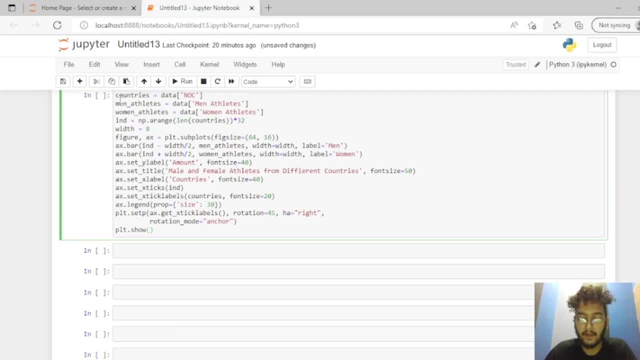 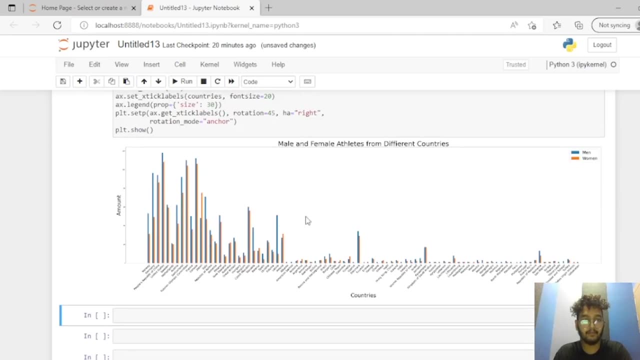 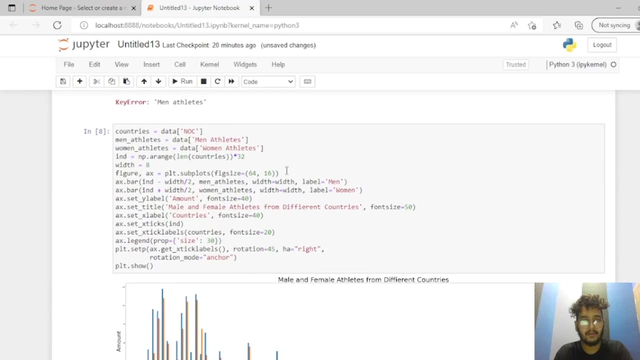 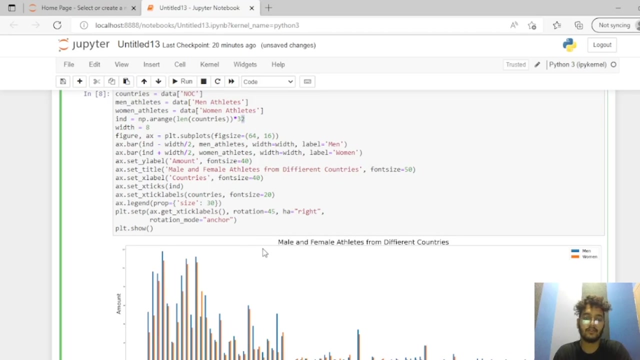 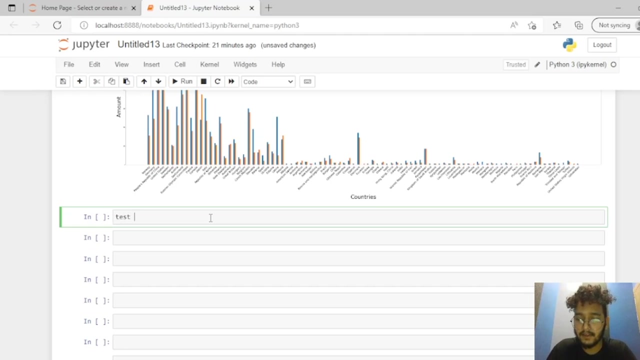 so, so press enter and so this is our bar graph. how looks like like for the how many countries? here we take countries, almost almost 32 countries. so this is our data for the 32 countries. so, moving forward, let's change our data now. so set test. 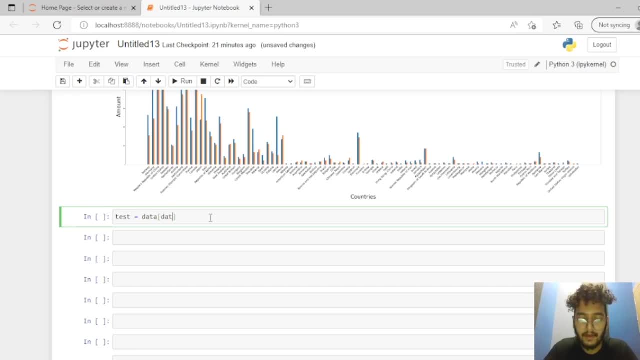 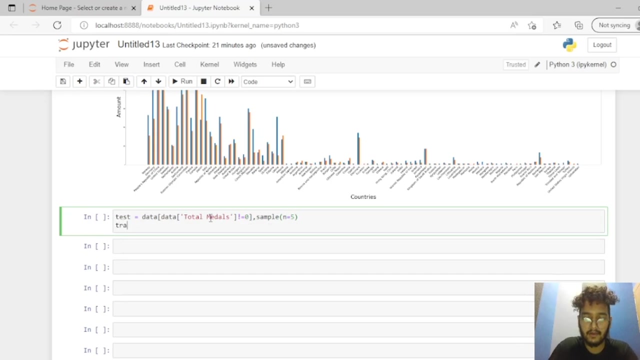 equal to data data data. so here, like total medals, like equals to, not equals to zero. so comma sample one equals to five. so we will write: train equals to data set, not solid data, only data. we have to write data data. second second we have to write here: 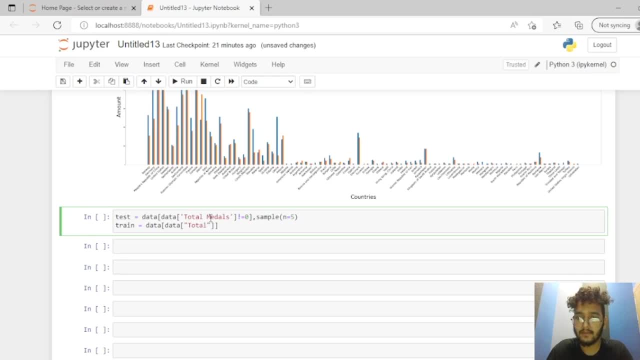 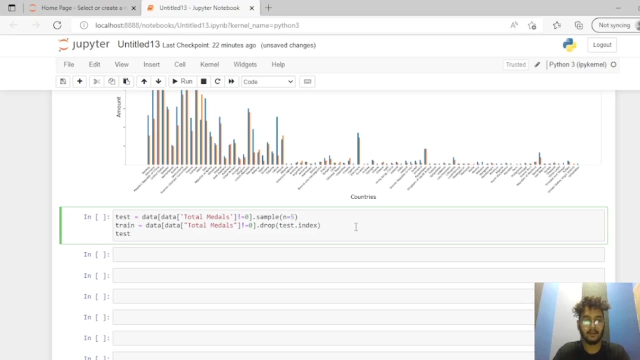 total, total, total medals. total medals: same same. here we will write drop, drop, drop. we will write drop test. we will write drop test. we will write drop test, dot, index, dot, index, index. so here we have to write dot. so here we will write test for testing data. 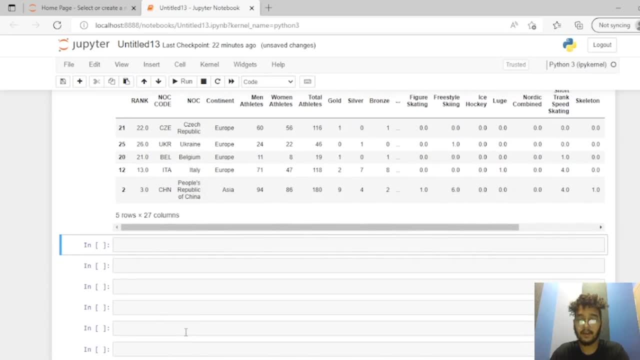 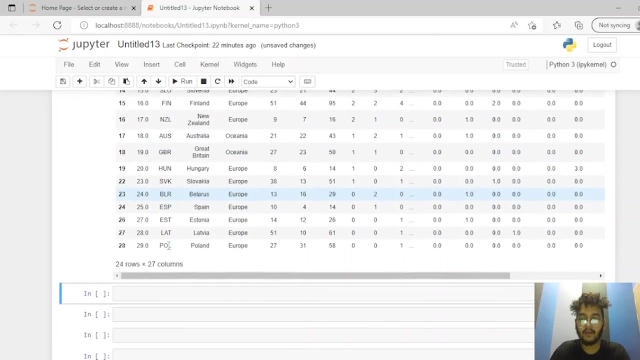 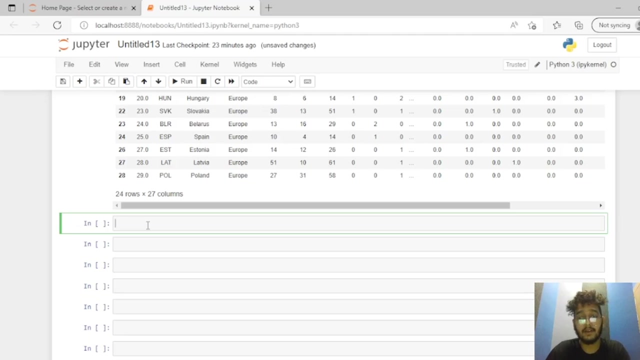 and press enter. so this is our testing data. so this is how the data looks like. and now write for the train data. so we will write only train, then press enter. so this is our training data. so now we will import sklearn, so we will write. so, like scikit, learn sklearn. 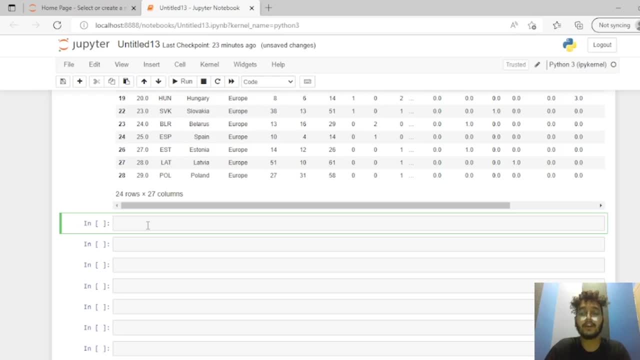 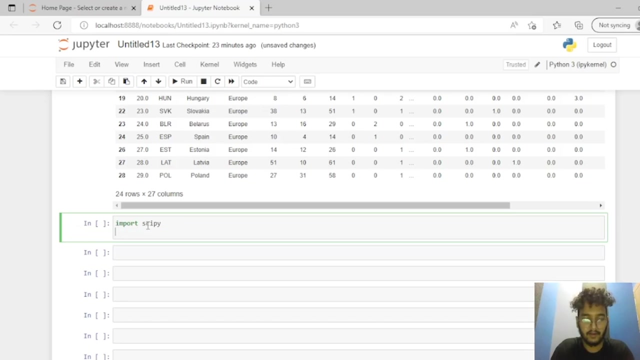 is the most useful and the robust library for machine learning in python, so it provides a selection of efficient tool for machine learning and statical modeling, including classification and regression. so we will write import scipy, will write import scipy, scipy, like from scikit learn sklearn dot svm. svm is for 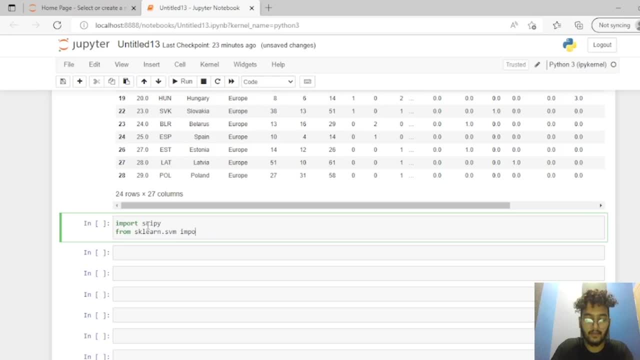 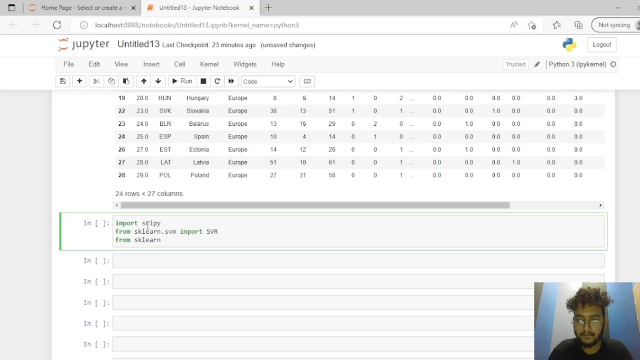 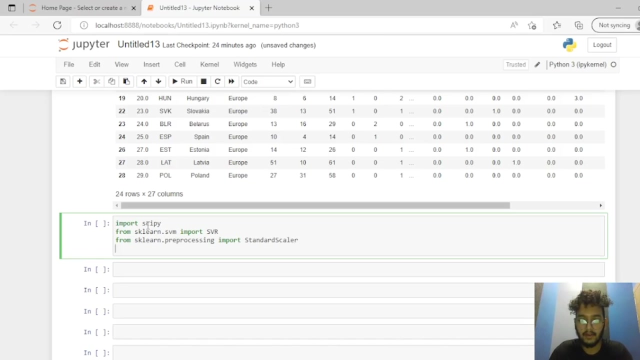 support vector machine and import svr. so this is support vector regression. so we will write here from sklearn dot preprocessing, preprocessing, preprocessing. we have to write import standard, standard, standard scalar, so like we have to write here from sklearn, from sklearn dot model, dot model. underscore selection. underscore selection. 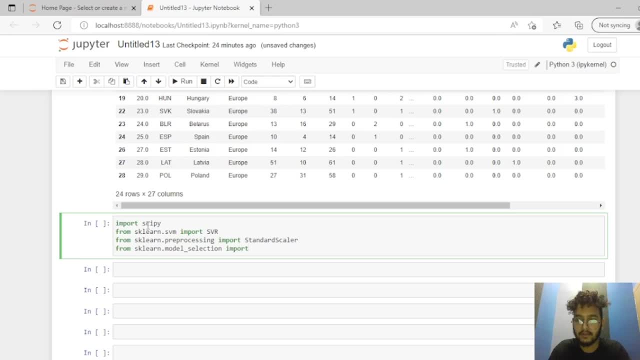 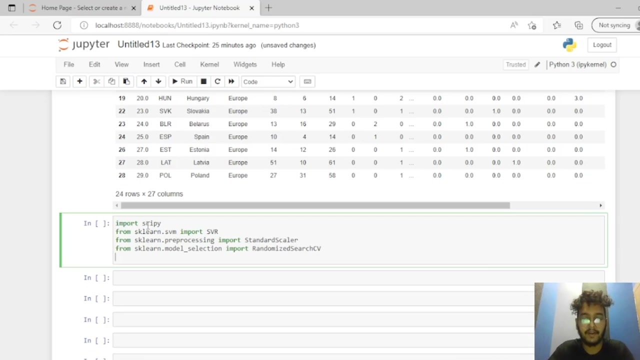 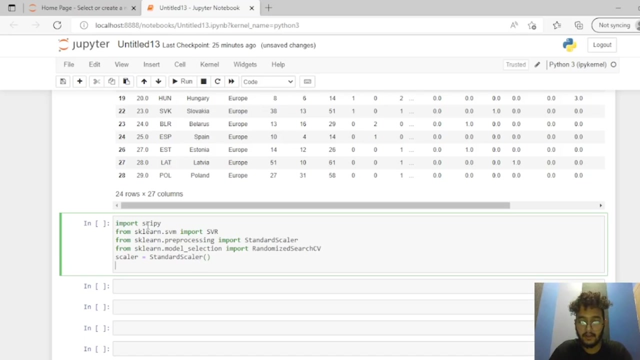 selection: import selection, import selection, import, randomized, randomized search search: cv c, capital c, capital, cv. so so let's get the our train data, and so let's get the our train data and the test data, so we will write scalar, scalar, standard, standard, scalar. and here we will write our 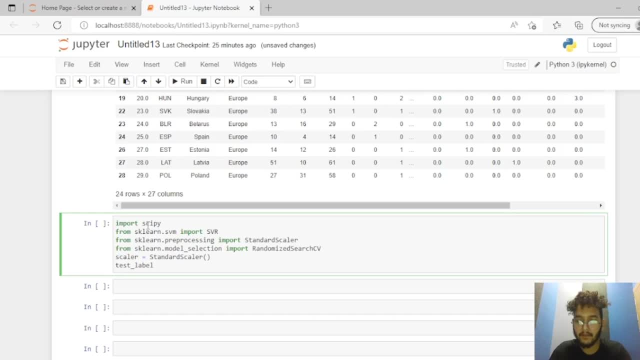 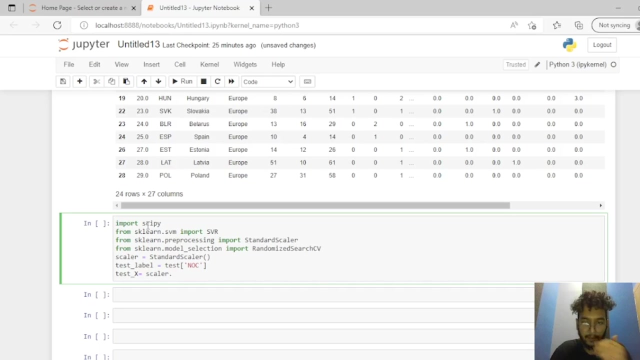 test label. label equals to test test. noc test test: underscore x. underscore x equals to equals to scalar, scalar. okay, my bad scalar dot dot fit underscore, underscore, transform transform test test test. test test: here two brackets and we'll here two brackets and we'll write right, right. 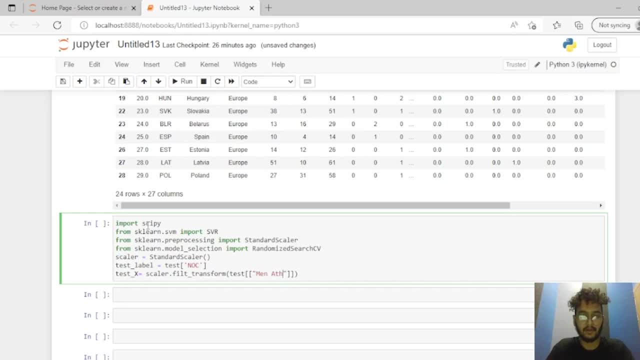 right, right, athletes, athletes. so comma, so comma: man man woman, man woman. So here we will write for the test: y-axis equals to test goal, silver comma. and the third one is branch, Branch. Let's enter Train label, Train NOC, Train underscore. 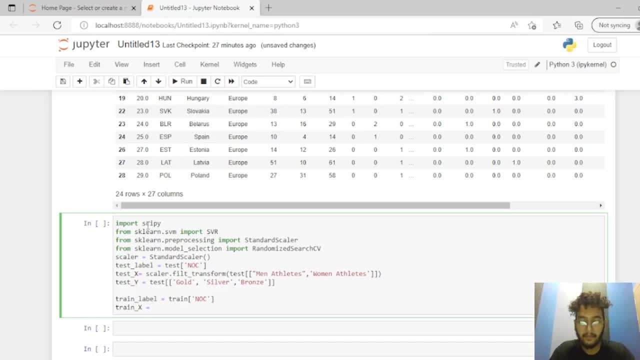 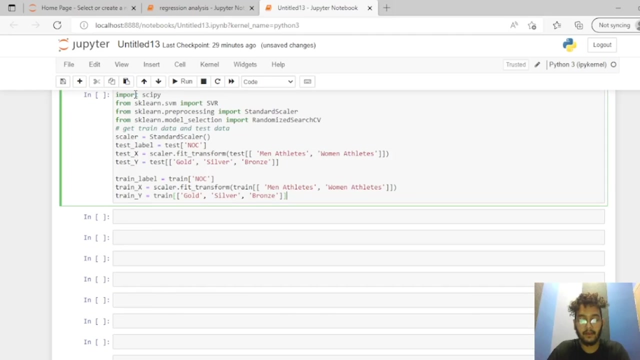 x equals to scalar dot fit, Like this Underscore transform for transforming the data. So we will write: train same athletes, athletes. train. underscore y equals to train. sorry, train underscore y equals to train gold comma, silver comma, launch, bronze, perfect and press enter. so now we will build our model. so we have to write: svr equals to: 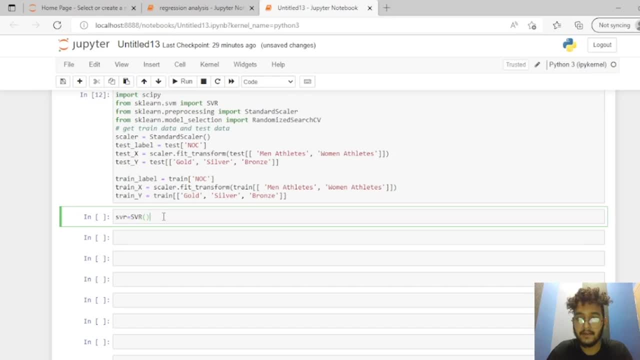 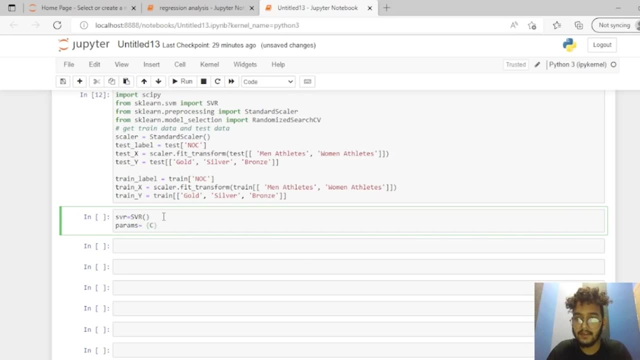 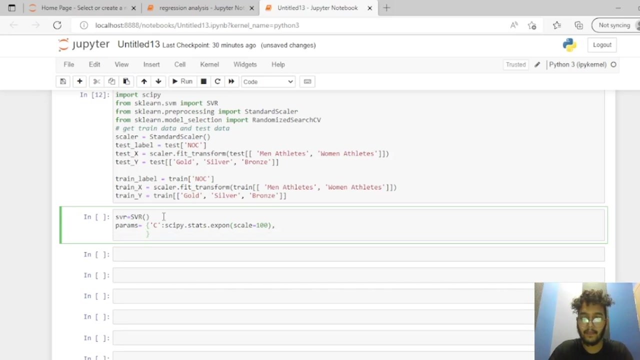 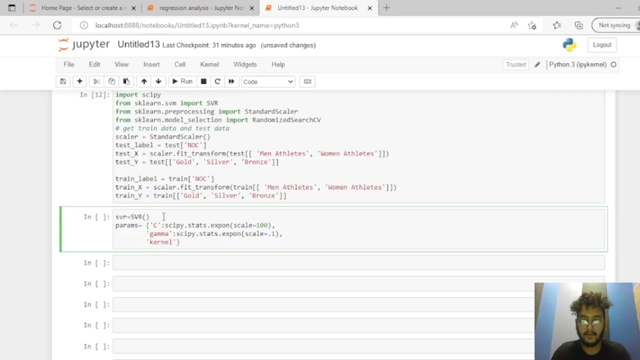 svr, like this: parms, for parameters equals to c, we will write scipy dot stats xp on exponential for scale: uh, equals to 100, okay, and we will use gamma, that colon: scipy dot stats 30. so here we will write: scale equals to point one, and okay, okay. so here we will write comma and the last one like kernel, so colon. 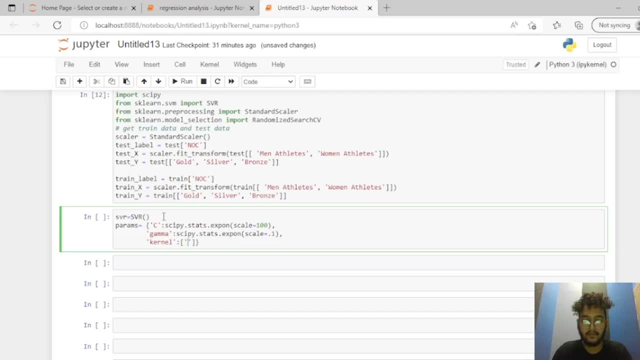 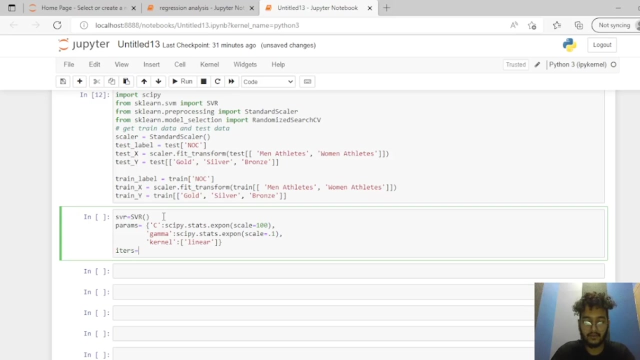 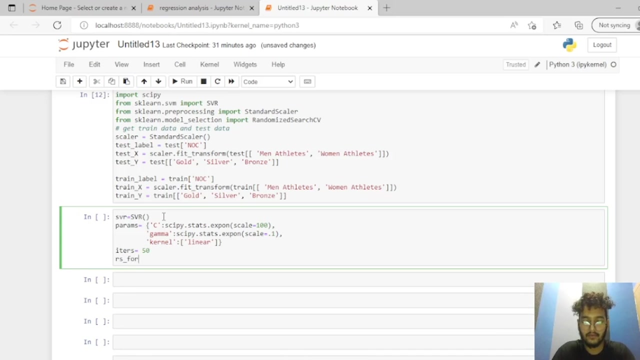 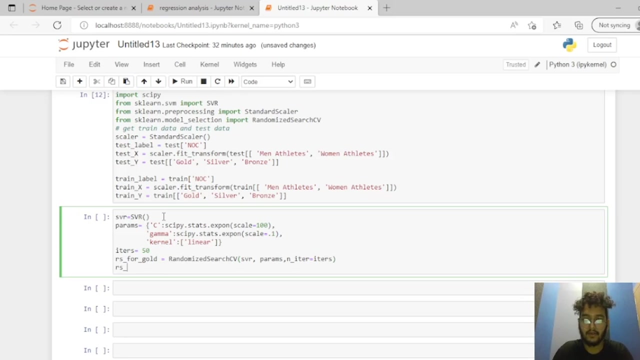 so here we will write comma and the last one like kernel. so colon, colon are running. handleも denier er, here let's can alt. can then Fran. randomized search: CER, comma, params, comma underscore. hiter equals to hiter. let's enter. we will write RS, or you have to write for same for silver and the. 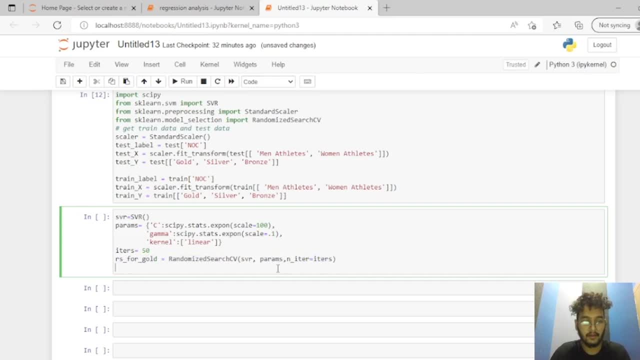 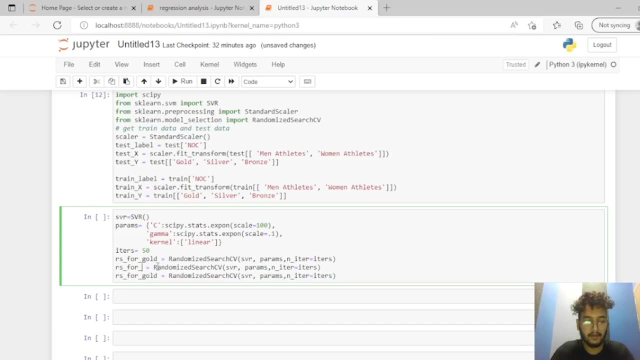 brown, so we can copy here and we can paste here again. we can paste here, so we will just change it. and here is: we have to write silver. you have to write for this. we have to write RS for gold dot bit, like now. we will train underscore X, label comma, train, train underscore Y, for this is we will do for. 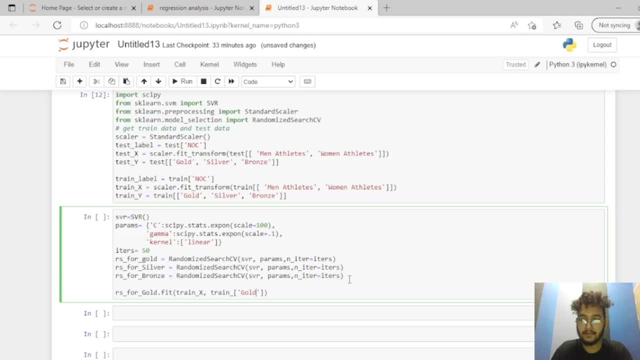 the train for this is: we will do for. the train for this is we will do for the gold, so so same. we will train this for gold, so so same. we will train this for the and the silver and bronze, so we can the and the silver and bronze, so we can copy here. so just, we will change here to: 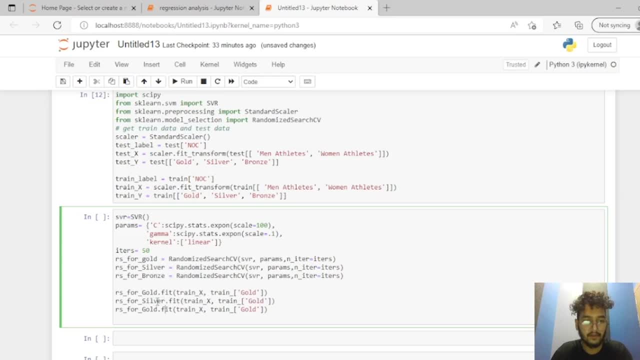 copy here. so just we will change here to silver here, sorry, silver here, sorry. silver here, sorry. and it'll add y underscore cold. and it'll add y underscore cold. and it'll add y underscore cold, underscore underscore good. gold dot prediction, sorry. predict train underscore x. so again, 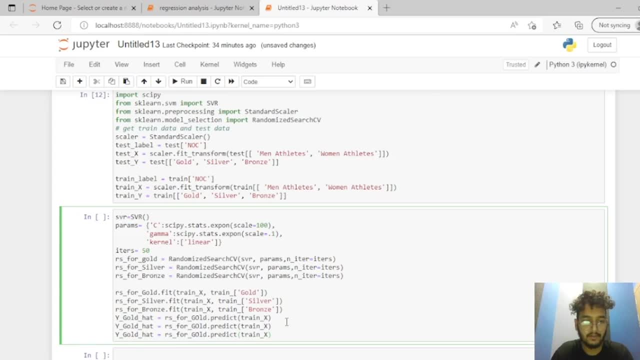 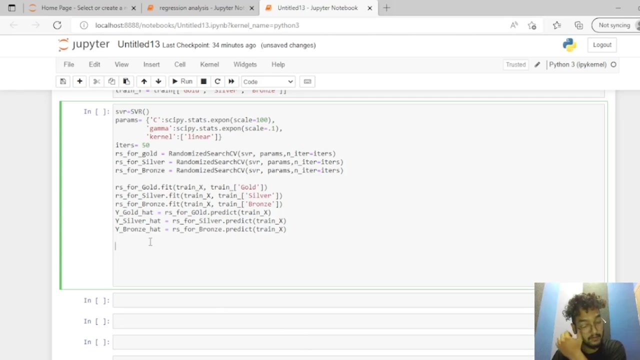 same for silver and bronze. so we will change it to silver. silver we will write bronze. so let's move our screen a bit up. so here we will write print pd dot data frame. so list, let's go set up zip and we will write y underscore gold, underscore head. 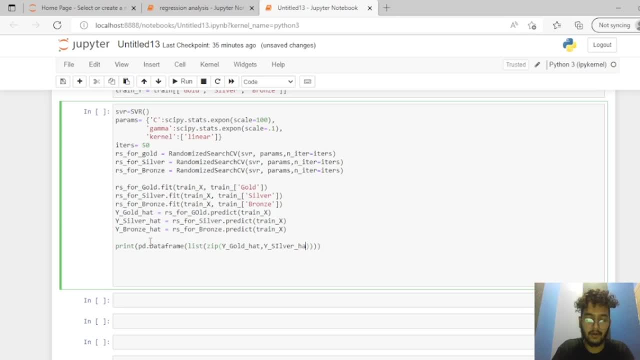 y underscore silver comma hat. okay, i small comma y underscore bronze underscore hat. we will write here: print: print train underscore y, dot reset underscore index drop equals to true here. so f i, g figure comma x equals to test underscore y, dot reset underscore index row to write here: test. 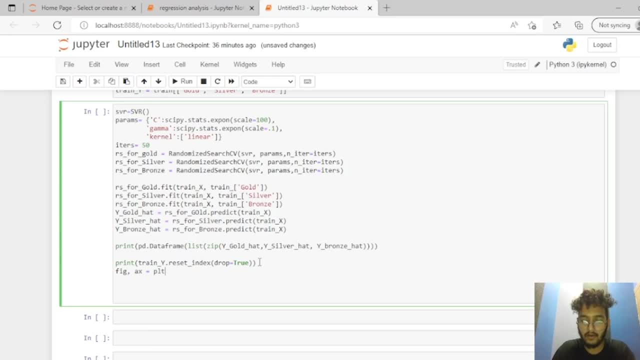 bad, sorry, sorry, sorry for this. we have to write plt, dot subplot. the plots we will make three by one. okay, so here we have to write: test underscore y equals to test underscore y, dot. reset underscore index. like captain, that's more all this is. so we will write here: drops. 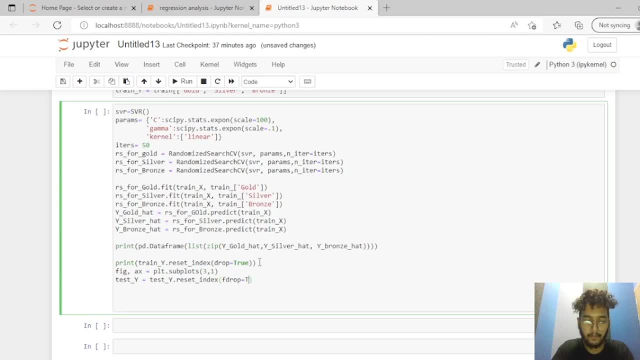 drop equals to through, so we will write here a 0 for 0 axis dot plot. so y underscore, gold underscore at then again 0, sorry, zero. and the color should be. color should be: let's take green, okay, okay, so again: ax, zero, dot plots, dot plot. 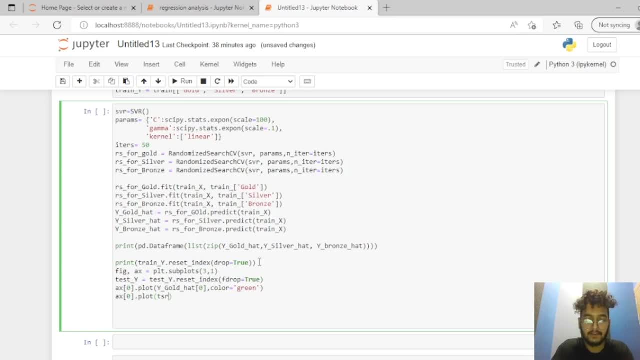 so here we will write test: what is test data test. underscore y square bracket, we have to write gold. okay, so the color should be. color should be blue. let's take blue here. so we will write blue, and we have to make for the same for the silver and gold brown. sorry, so we can copy paste here and we. 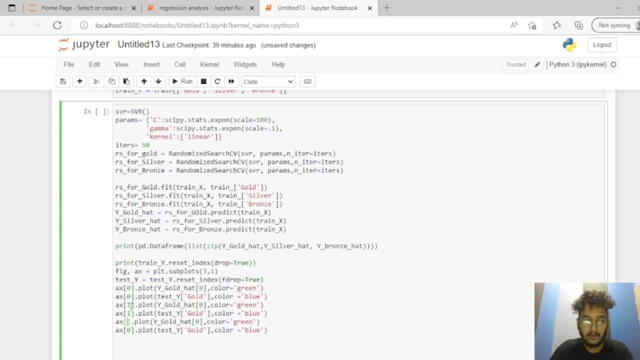 can give the different axis name, this will be two. so here we have to write one, two. let's write silver two, two, Okay, here, silver 2,. here we have to write bronze. we have to write bronze. So the time has come. we have to write plt dot 2.. 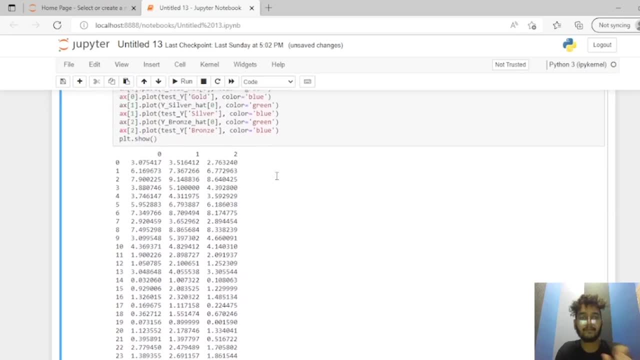 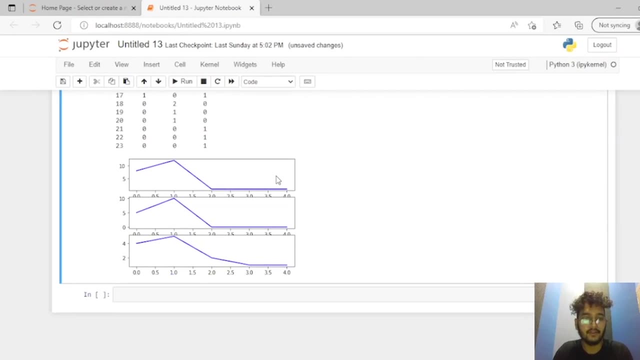 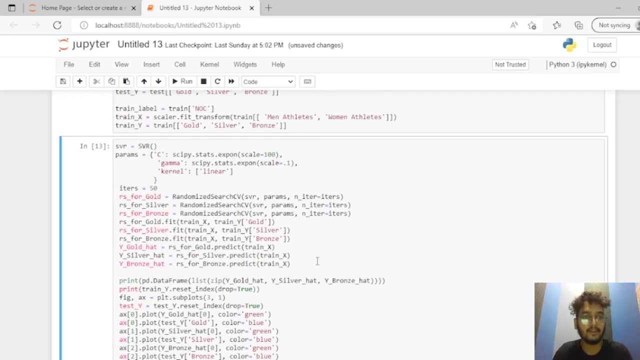 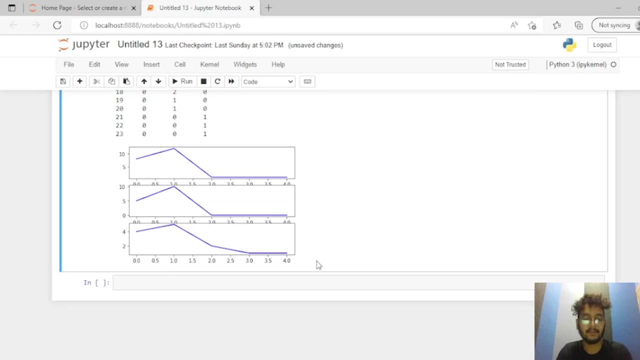 Now press enter. So after pressing. so our model. So this is how the SVM regression looks like. So this is how we made regression analysis using SVM. So moving forward, let's see some job opportunities in regression analysis, An extremely potent statical tool. regression analysis. 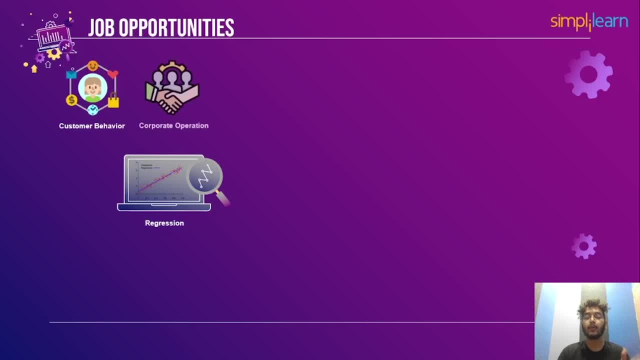 Regression analysis can be used to get insight into customer behavior, corporate operation and factor affecting profit. Businesses can use linear regression analysis to analyze trends and generates estimate or forecast. A product sale also be examined while using regression analysis. For example, McCain Erickson India Private Limited advertising company used linear regression. 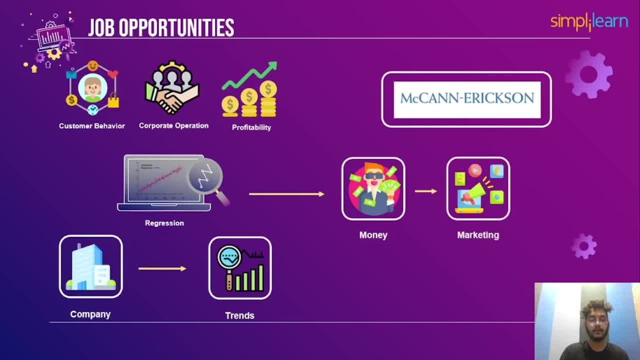 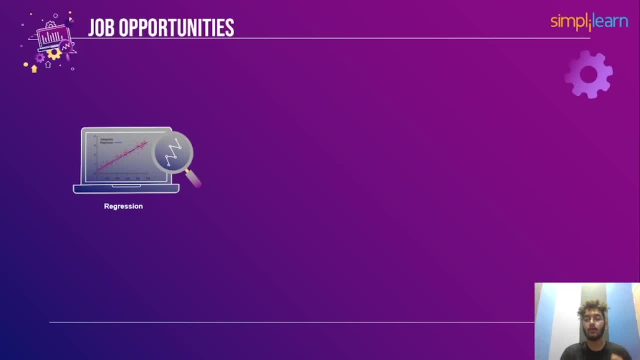 to determine if the money spent on marketing or a certain brand resulted in a significant return on investment. The benefit of regression analysis is that it allows us to control the variables that can affect sales, while also capturing the individual effect of each marketing effort. In the real world situation, several advertising campaigns are active at the same time. 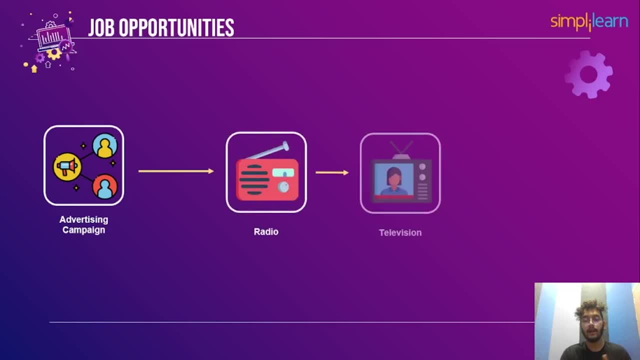 If two campaigns are broadcast simultaneously on radio and television, a regression analysis can capture both the individual and the combined effect of running these ads together. So The impact of regression analysis can really hold a huge potential to generate significantly high productivity growth. Currently, one of the fields with the greatest soul of growth is analysis. 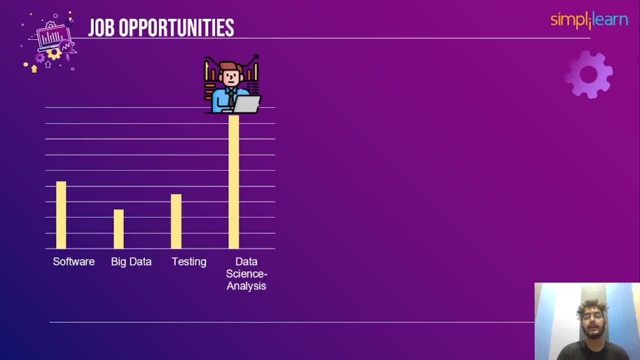 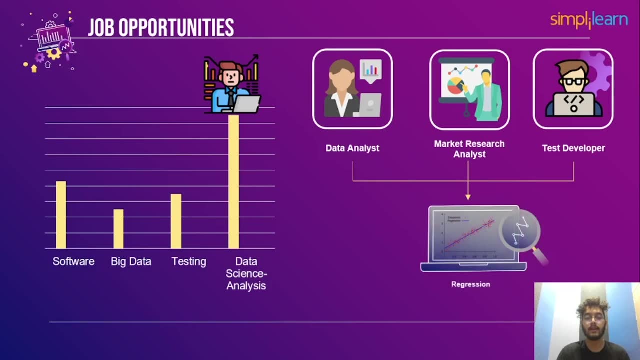 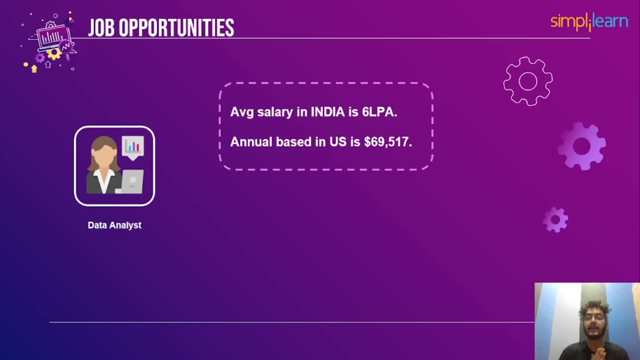 Analyst engineers are in high demand. There are various job profiles like data analyst, market research analyst, performance as developer and many more who are hired with a skill of regression analysis and machine learning. The average salary of data analyst engineers in India is 6 lakhs per annum and the annual 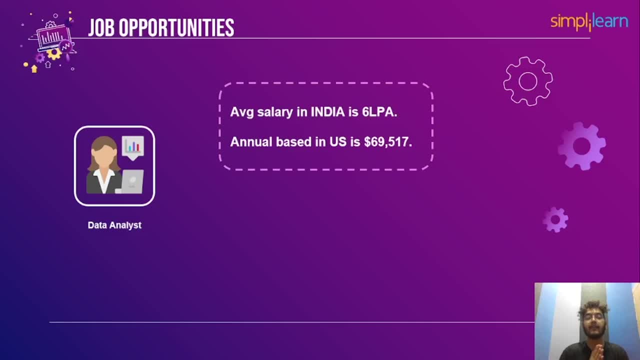 base pay for US data analyst engineers is $69517.. All ventures as of now have countless uses in regression analysis, which is the fundamental inspiration behind why there is an interest of occupation in that field. The growth in technology has led to increasing demand for the professionals who can understand. 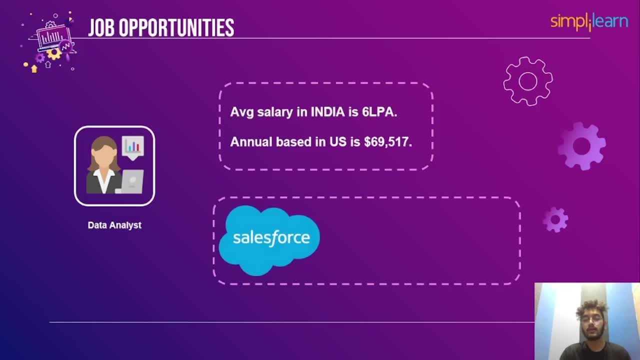 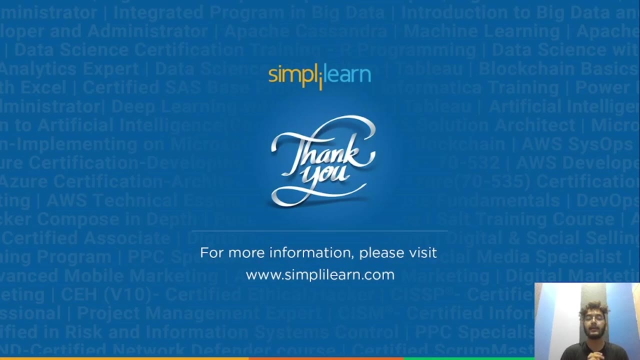 and use vast amounts of data. Companies like Salesforce, Google, IBM and many more are constantly hiring analyst engineers. I hope you guys found this video informative and helpful. If you have any doubts or feedback, feel free to leave them in comments below. 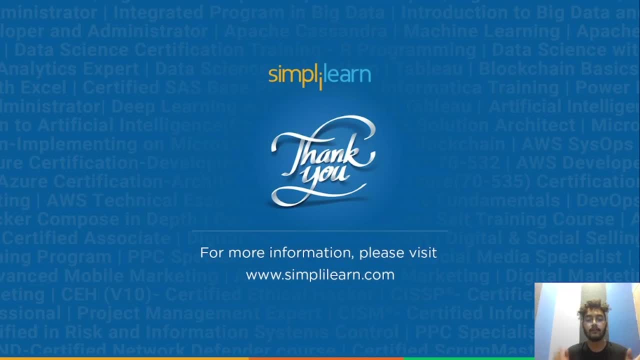 We will be happy to help you. Machine learning is a trending field with a bright future if chosen as a career. Here is a machine learning certification course: by Simply Learn to become a certified machine learning professional. Kindly check the course details from the link in the description below. 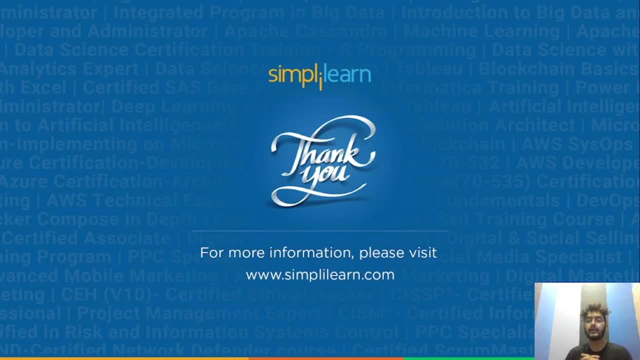 If you like this video, please subscribe to our channel and don't forget to hit the bell icon. Keep learning.